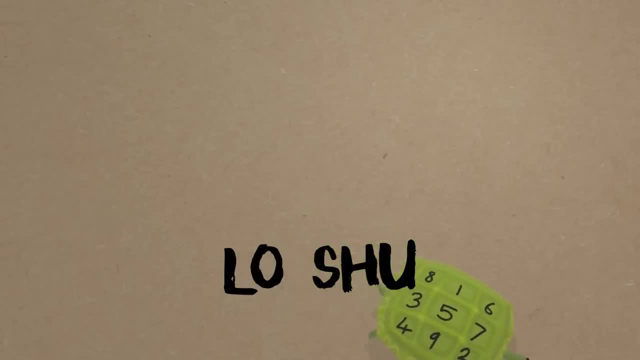 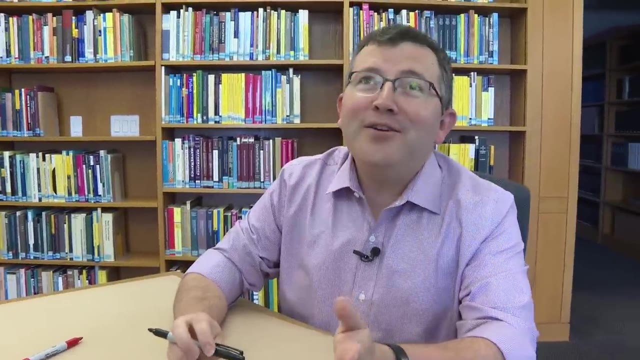 I know there are lots of other magic squares. We're going to talk about them shortly. Yeah, Is a magic square still a magic square if any number is repeated, Or is that kind of imperfect I? so I would argue that those are imperfect magic squares And in fact that's kind of what. 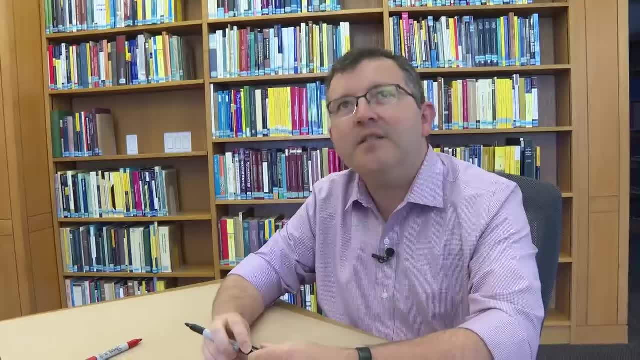 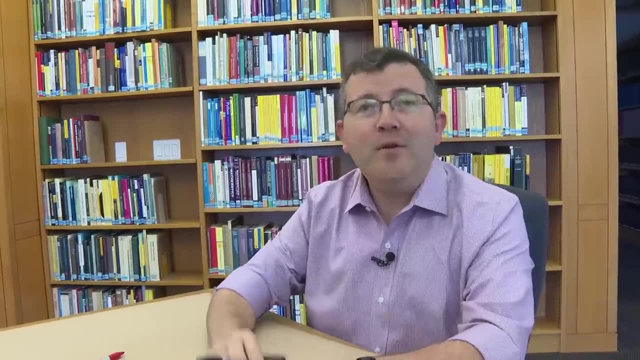 makes it hard, I think, to find magic squares. If you allow repetitions, you know you can really find magic squares quite easily, right? I could just repeat all the numbers here, right? Just take your favorite number. Mine is 19.. I think it would be nine, but nine is not prime, So it's 19.. 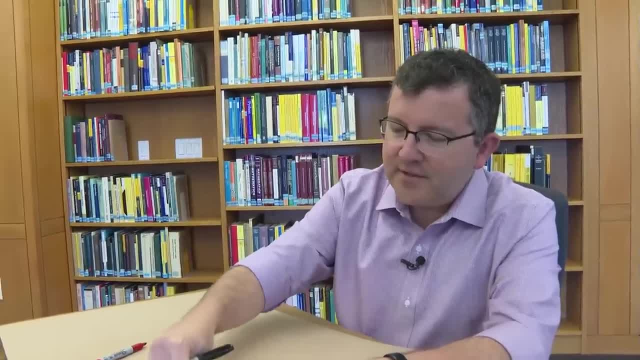 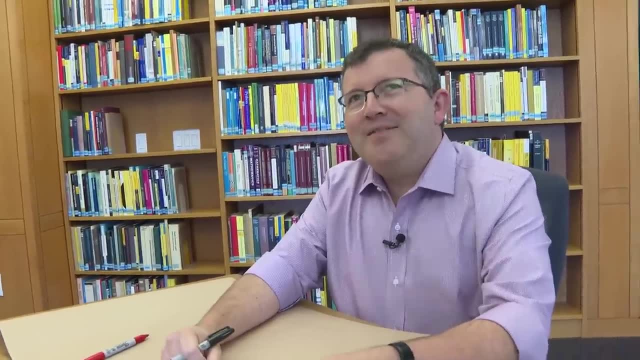 So if I put 19 everywhere in these nine entries, I'll just get a magic square that way, But it feels like it's not. it's not a magic square. It's not a real magic square. It feels like a fake magic square. So what I want to do is look at 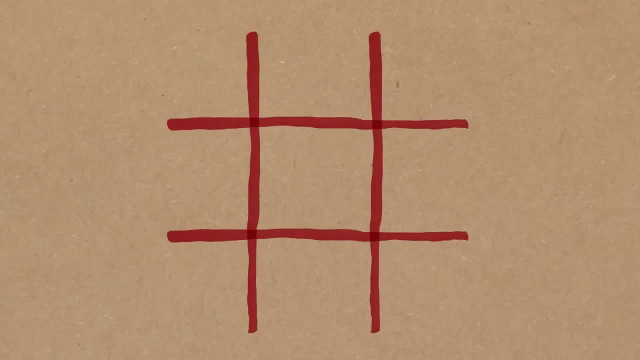 three by three magic squares. but I want to impose one more condition, which is that I want the entries themselves to be the squares of numbers. So I'm going to draw for you an example of this, and it'll be a bit of a cheat People who've been seeing Numberphile videos for a while. 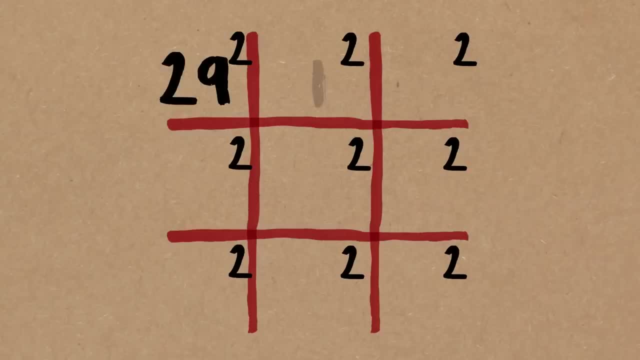 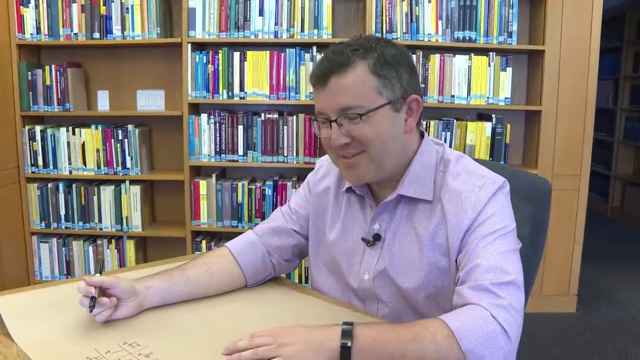 are going to recognize this. So this is: 29 squared, 1 squared, 47 squared, 41 squared, 37 squared, 1 squared, 23 squared, 41.. 21 squared and 29.. And this is a very famous magic square and it was made famous by Numberphile. 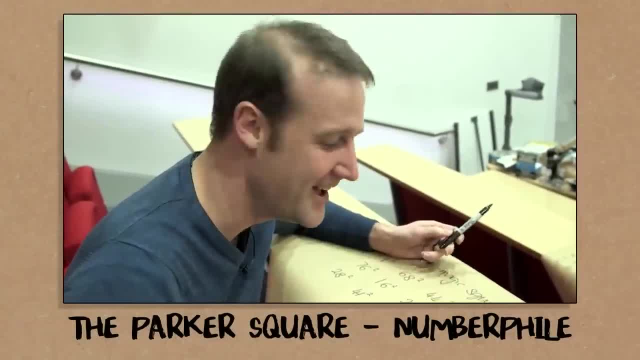 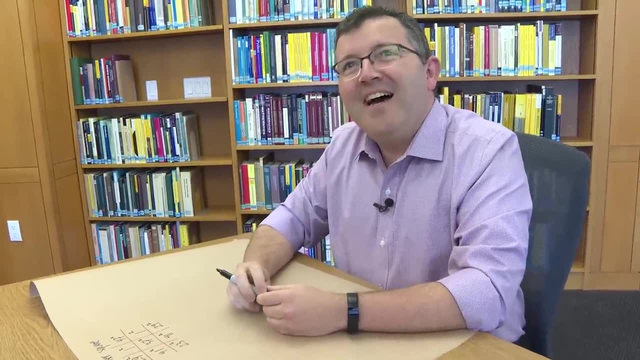 So this is the Parker Square, So I'm not calling it the Parker Square. Matt, you know what this video is called. I'm calling it. oh for crying out loud, This was famously Matt's attempt at all squares. That's right. That's right. It's a very good attempt. I think this is a very reasonable. 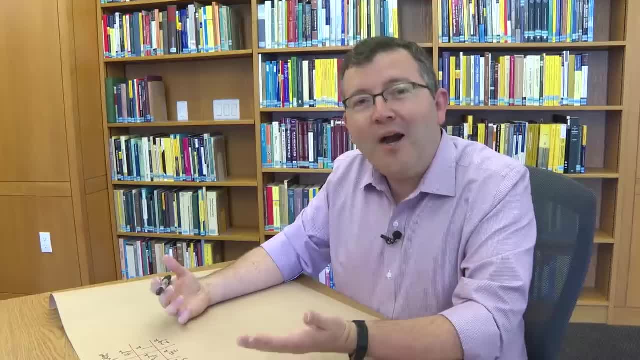 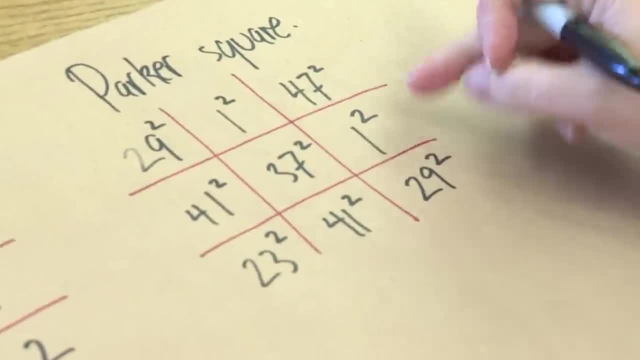 attempt. In fact, it complies with almost all the requirements of a magic square, of a magic square. So every single entry is a square number right. And it's true that if you add up all the rows and all the columns, 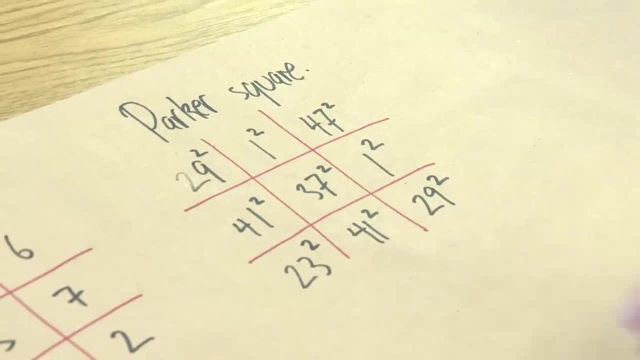 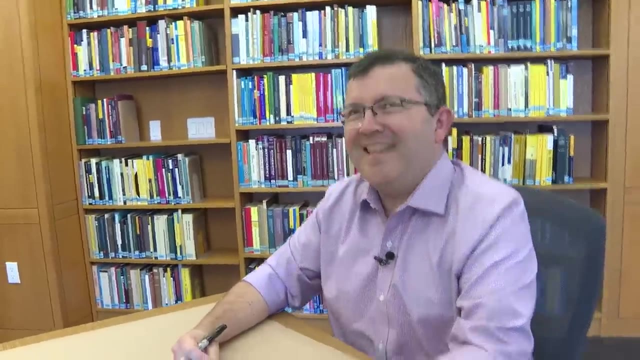 and if you add up the two diagonals, it all adds up to the same number, So it satisfies the main requirements for being a magic square. Doesn't one of the diagonals fail? Wait, sorry, Can we check that? This diagonal here works? This diagonal here doesn't work. 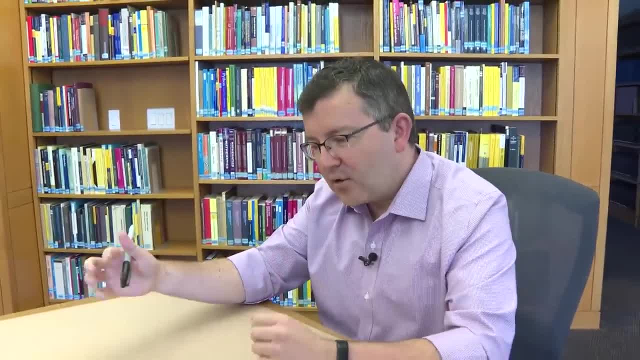 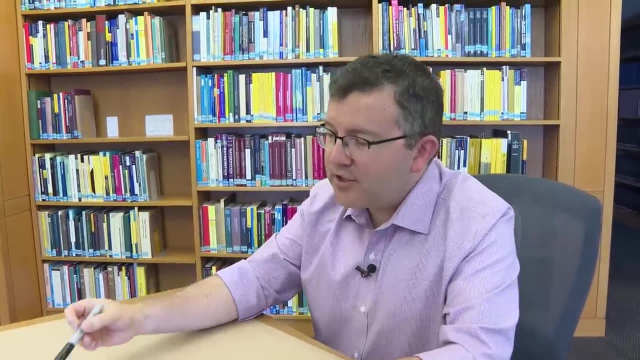 One of the diagonals does not, and so in that sense it's not quite a magic square of squares. It's one of the main requirements for being a magic square. It's what people tend to call a semi-magic square, And there's some repetitions of the entries. 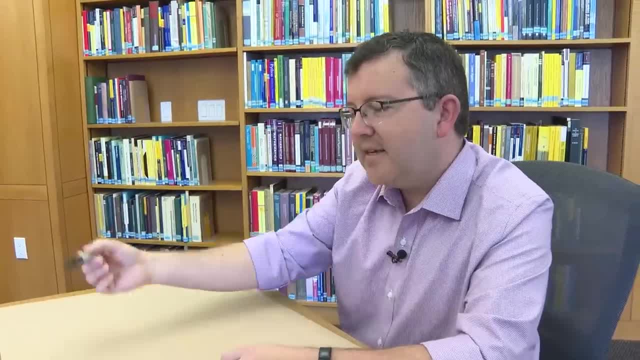 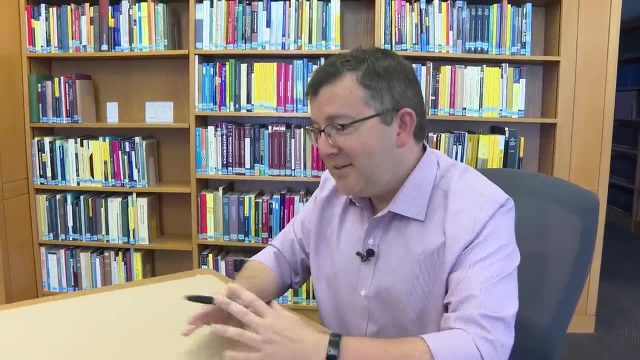 So, for example, you see the two ones here, you see a couple of 29s, a couple of 41s, And so it sort of feels like it's cheating just a little bit, but it's a really good attempt, So it's a good starting point. 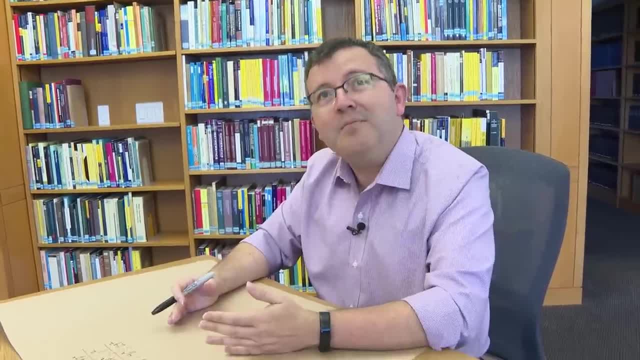 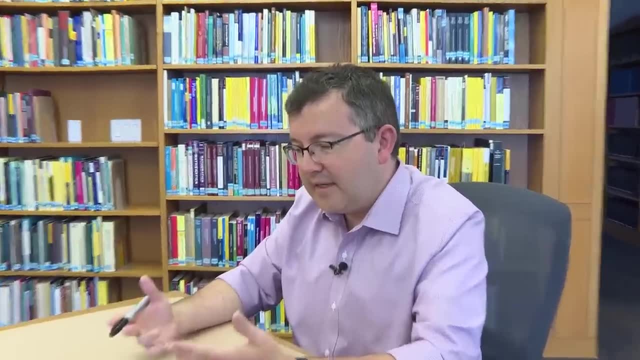 Sometimes in math, when you can't solve a really difficult problem, you try to solve a simpler problem And making some of these, allowing some of these entries to be the same- as a way of trying to simplify the problem in a way that might use some interesting mathematics as well. 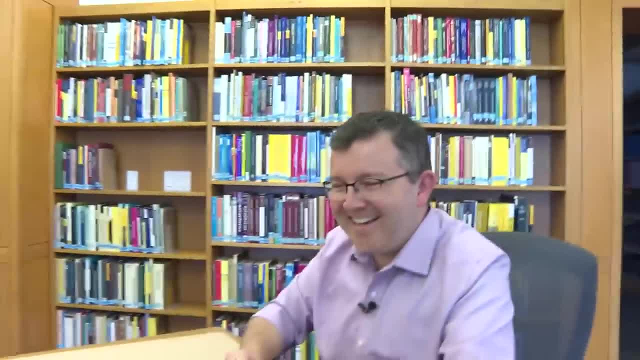 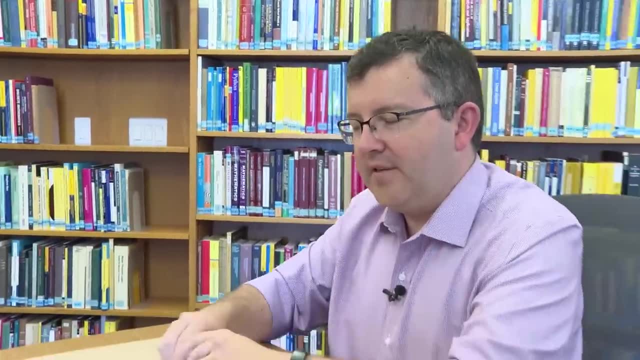 Okay, Parker Square: Great Good attempt, Yes, Okay. so there are a couple of other squares that I want to show you, Because so, as we saw in the Parker Square, there's just a couple of things that aren't quite right. 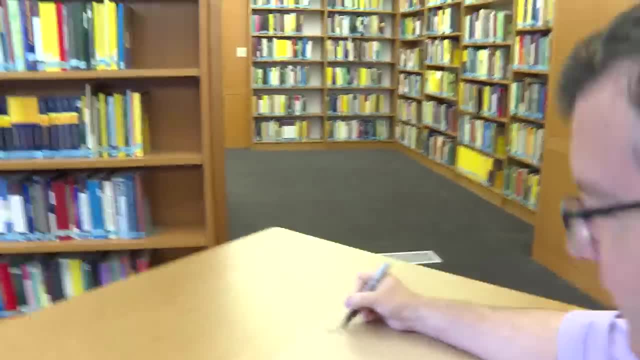 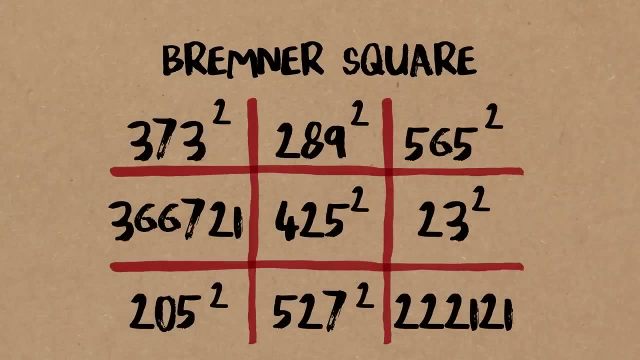 And there are some really famous ones. These are sort of from the late 90s, So one of them is called the Bremner Square. Okay, this is a big one, Okay. so this is another attempt at a magic square of squares. 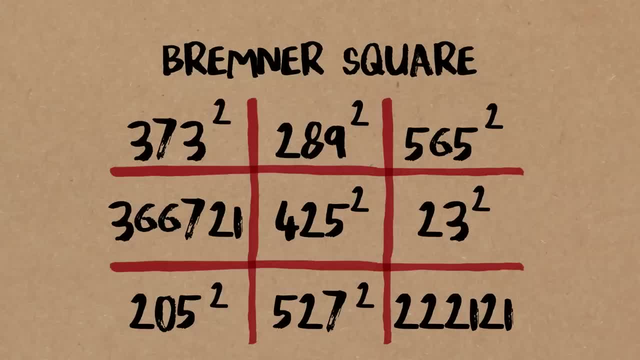 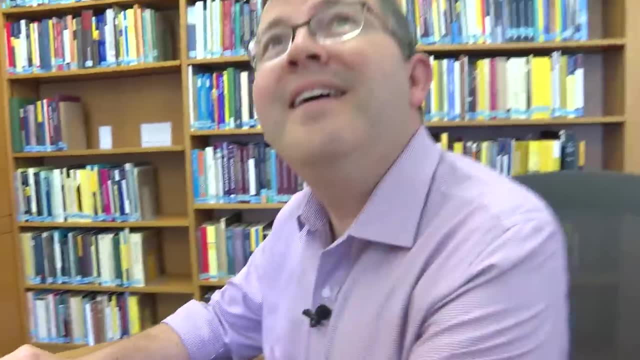 And it's very good- In sort of a different way from the Parker Square. This time, you'll notice almost immediately that there's two entries that are not squares. That's where this fails. That feels like an even more fundamental failure to me. 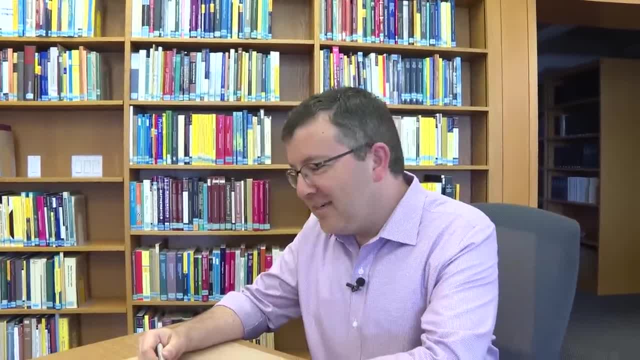 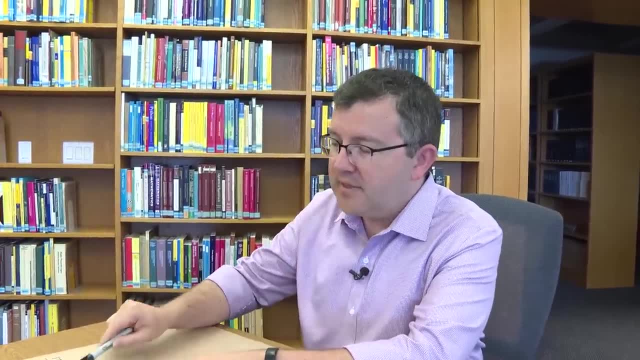 Yes, Are they close to being squares? Not really, I don't think. It is a little bit sad that they're not really squares, But what is true here, though, is that the columns and the rows and both diagonals are up to the same thing. 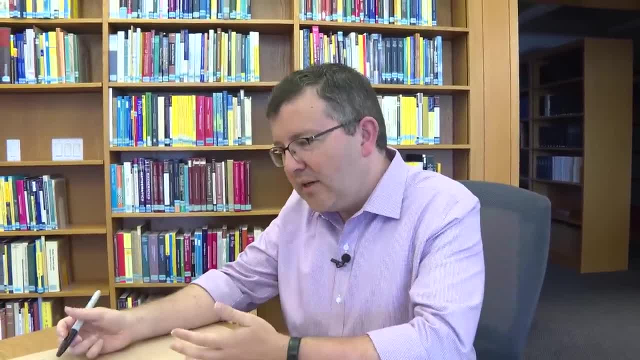 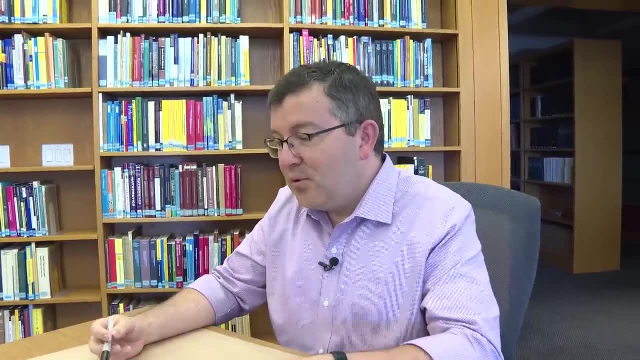 So somehow we managed to at least preserve that property. But then we broke the squares. We do have distinct entries. So you know, you're sort of you feel like you're making progress. I mean, it'd be, you know, cool to have one that had like eight squares, you know, and maybe only one that's not a square. 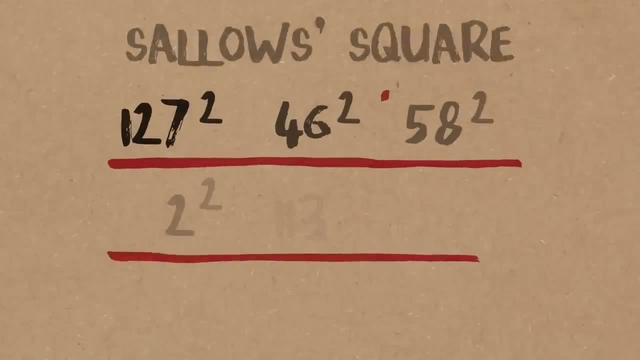 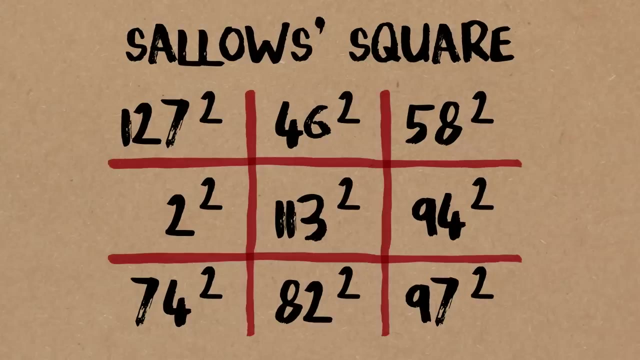 I don't know of one And I'm not sure if one has been found yet. There's another square consisting of square entries which is almost a magic square. It's a semi-magic square, It's by Salos And in a sense it's sort of an improvement on the Parker Square, in that all the entries are distinct. 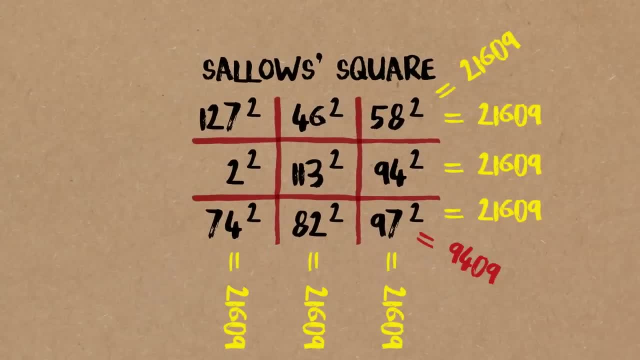 However, just like with a Parker Square, one of the diagonals doesn't add up to the same number That all the others add up to. That feels like one of the best attempts so far, doesn't it? That's right, Yes. 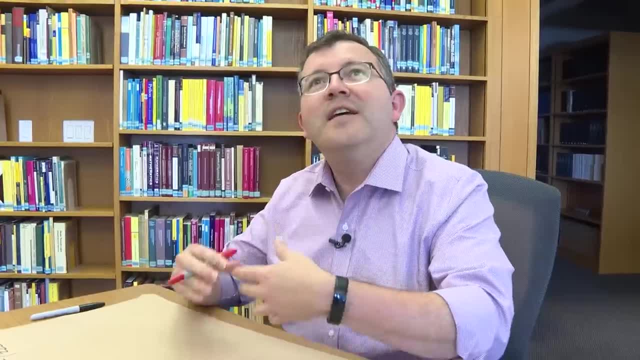 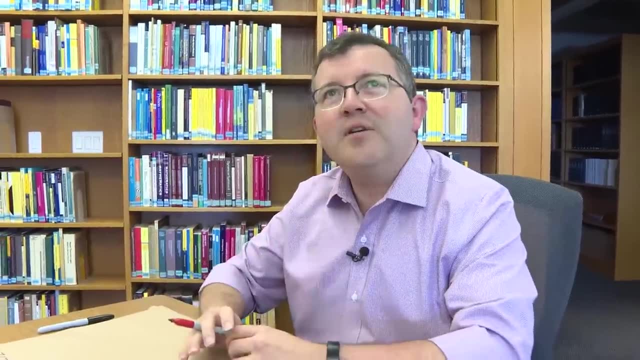 In fact, it's really nice that if you just remove one of the conditions, then you really can find them. It's a very difficult problem, precisely because of how all of the conditions come together. Of course, this is a fundamental question here. 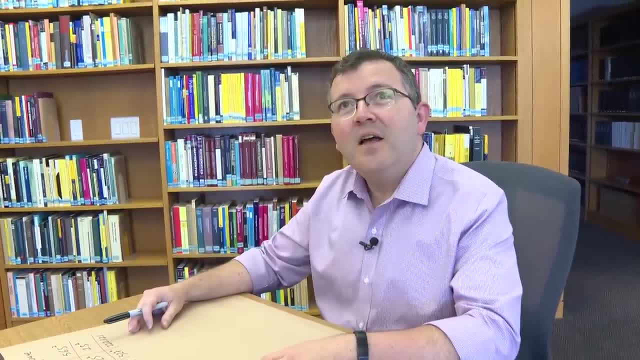 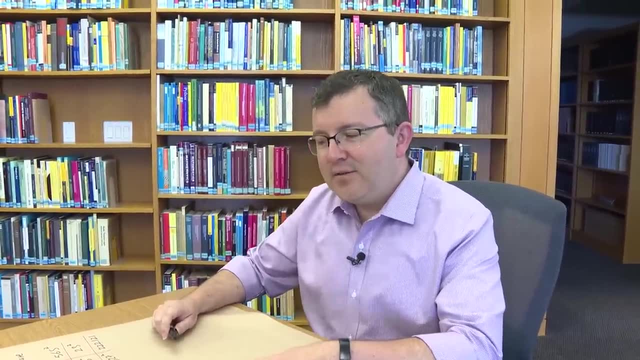 Does one exist? Has anyone ever found a magic square of squares? As far as I know, no. It's really sad And in fact what I want to do today is try to convince you that there probably isn't one. So I know that's sort of a sad thing to say. 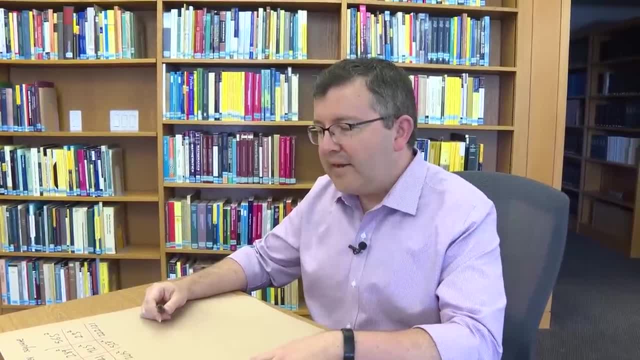 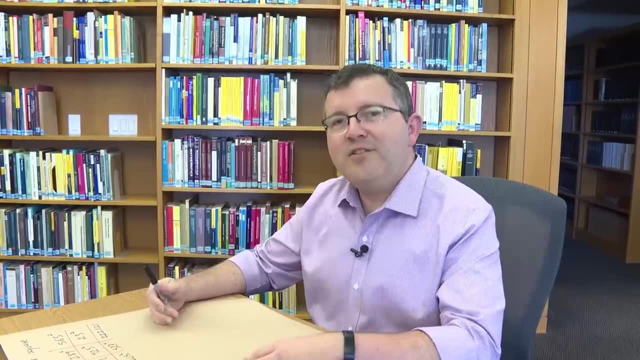 I would love it for it to be a magic square of squares, But I think geometry is giving us a bunch of indications that this just might not be the case, And so, in fact, what geometry suggests is that if there is a magic square of squares, 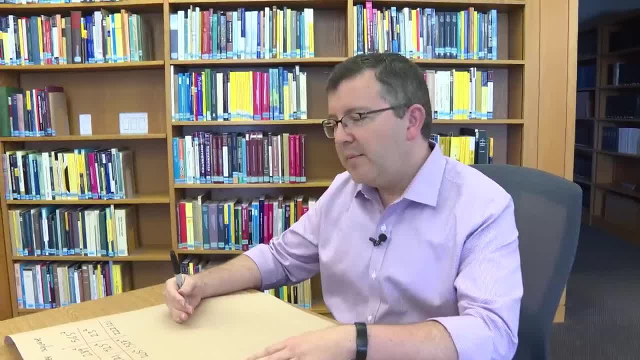 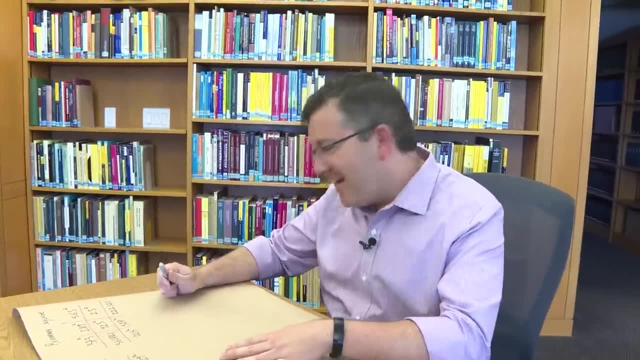 it's going to be really, really difficult to find, And it's sort of beyond what we can do by just trying small things. This doesn't look like geometry to me, Right, Right, Oh, my god, yes, Thank you for that question. 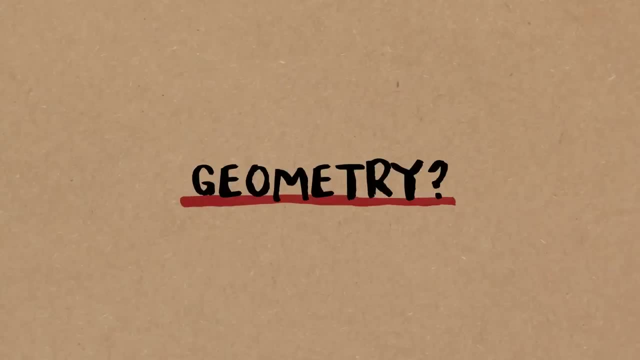 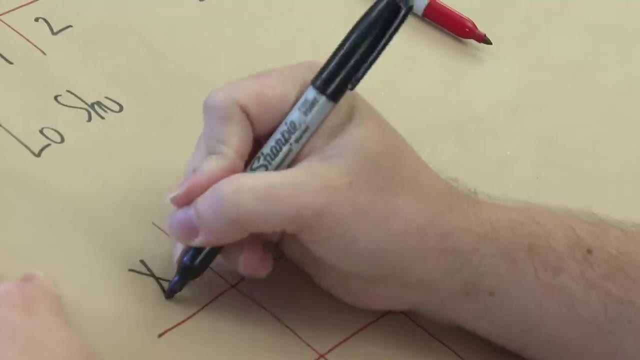 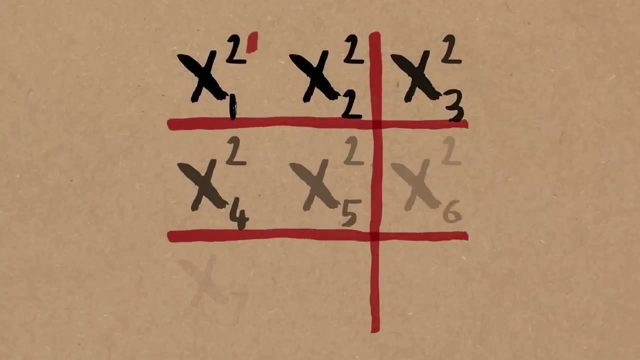 Yeah, Let me try to show you where the geometry at least starts coming up. Let's do it. So we're trying to find nine numbers, each of them a square, And so I need to give them names. I'll call them x1 squared and x2 squared and x3 squared, and so on. 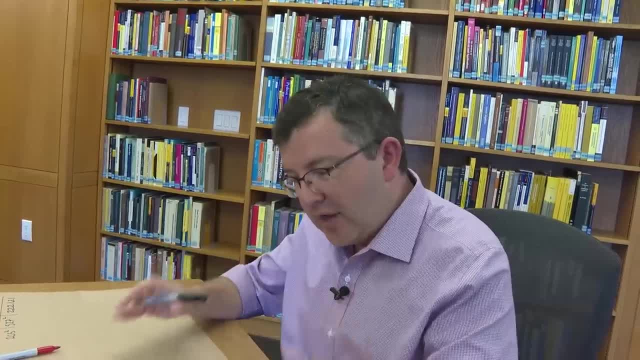 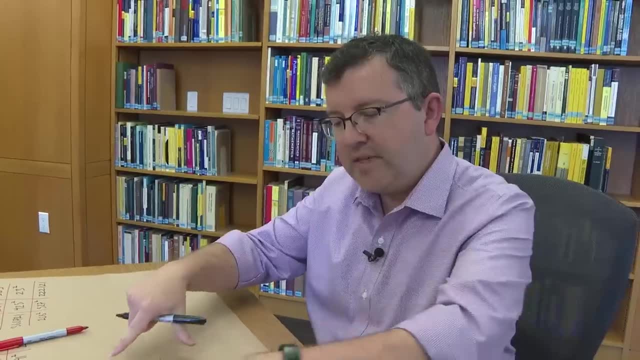 What we're hoping for is nine distinct positive integers- x1 through x9, that I can put into one of these 3 by 3 grids in such a way that the rows, the columns and the two diagonals add up to the same number. 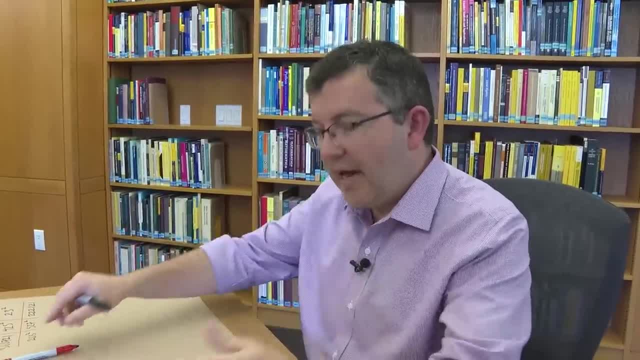 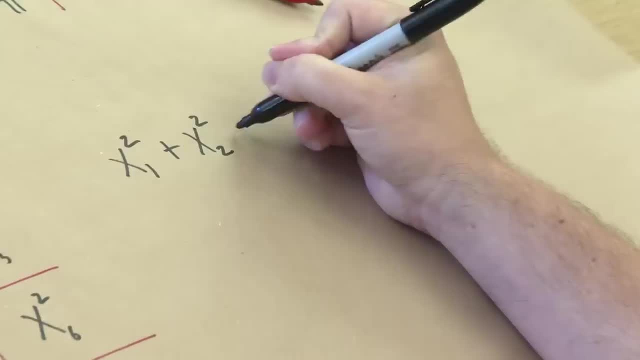 And so I can actually write out what those conditions are in terms of just algebra. It's like a monster equation. Yeah, It's going to be a set of monster equations, in fact. So let me show you. So, for example, I need to know that the sum of the elements of the first row is equal. 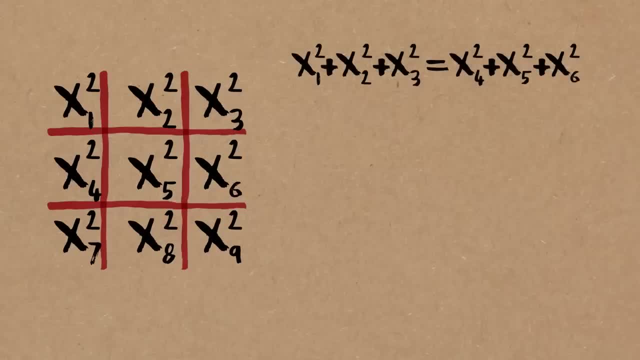 to the sum of the elements in the second row. So I can just write out this monster equation. I also need the same two sums to equal the sum of the third row, So I can write another equal sign here. This all has to be the same. 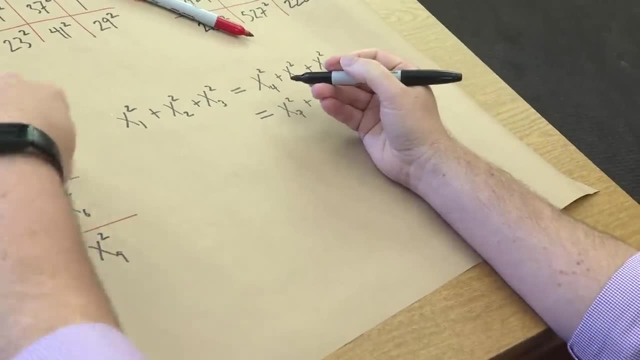 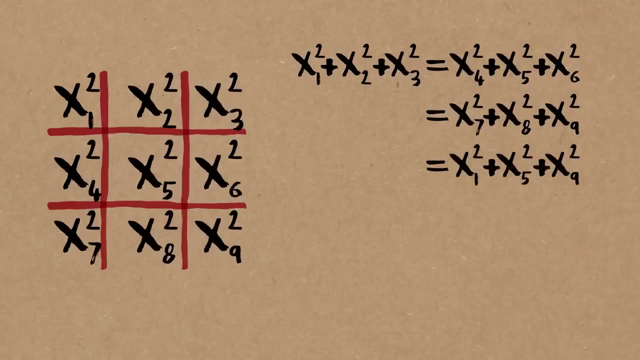 OK, I also need to know that this sum is the same as the sum of the two diagonals. So let me do those next. So there's x1 squared plus x5 squared plus x9 squared, And then the other diagonal, so it'll be x3 squared plus x5 squared plus x7 squared. 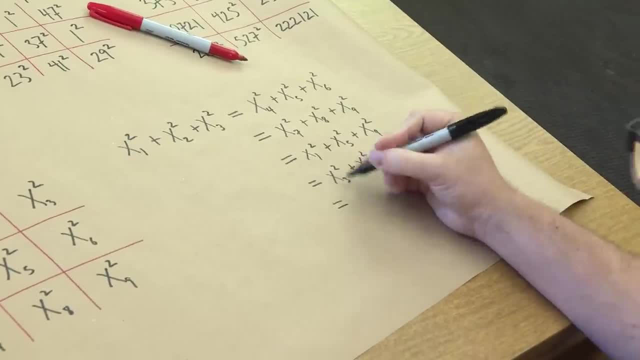 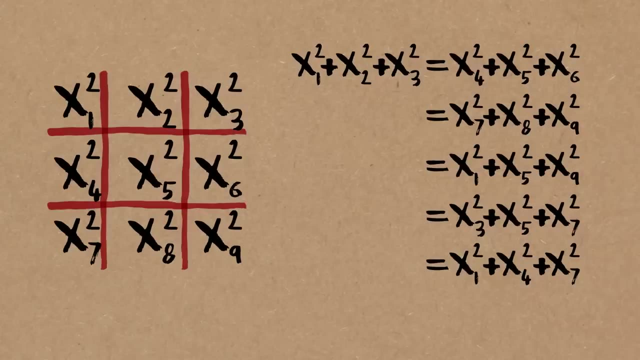 This is a bit messy, But we still have to do the columns. So the first column will be x1 squared, And then the second column will be x2 squared plus x4 squared plus x7 squared, And then I'll do the second column: x2 squared plus x5 squared plus x8 squared. 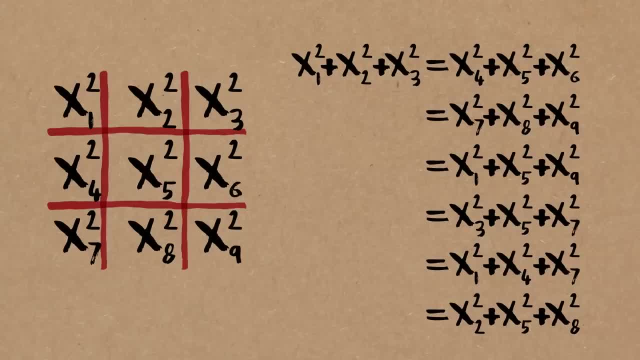 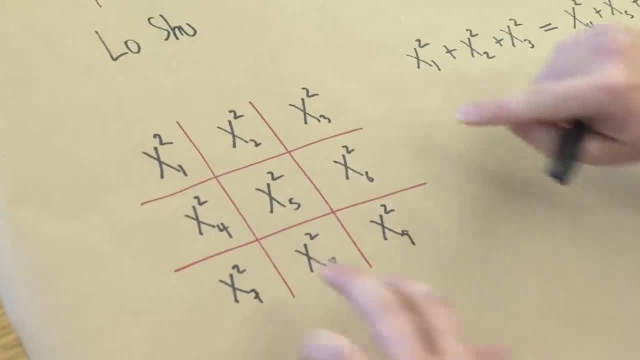 OK, And I'm still missing the third column. OK, But here's something. This is a really important observation. So once I know that all three rows add up to the same number and the first two columns add up to the same number, that forces the last column to add up to the same number as. 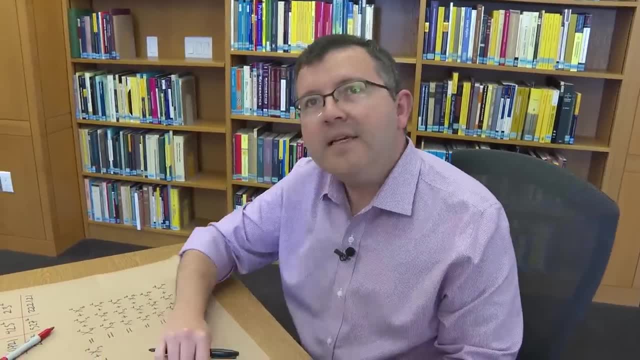 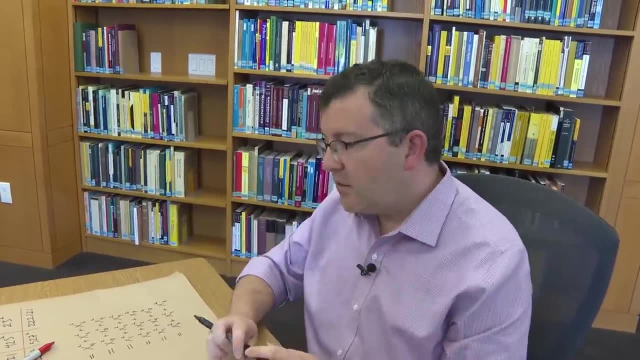 all the previous rows and columns, Right? So this is not a condition that we need to sort of set out, because it's already implied by all the other ones that we have imposed. So this is sort of an important thing because it cuts down on the number of equal signs. 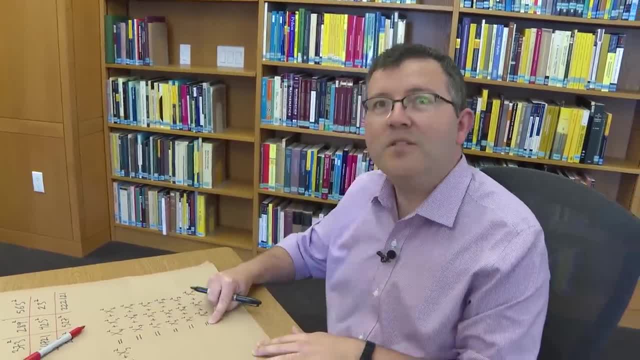 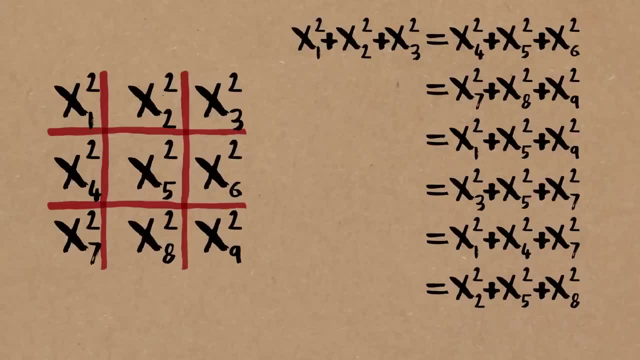 that I've written. OK. So there's only one: two, three, four, five, six equal signs. I don't need one more equal sign to say that this is all equal to the sum of the last column. That's an important geometric point. 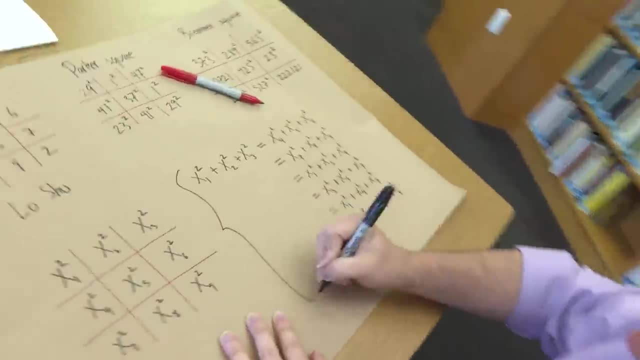 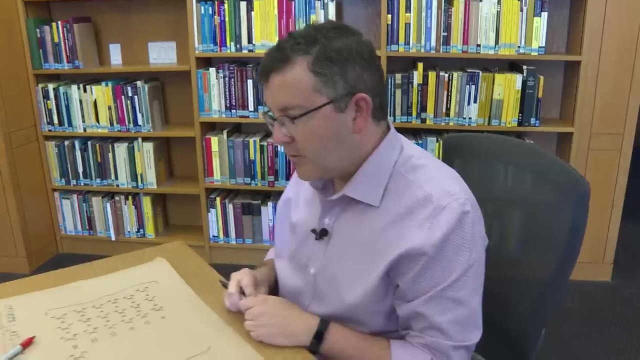 OK, So we have a mess here, So we have this like huge system of equations, OK, And so I need to make sort of a few observations about this system of equations. OK, What I want to try to argue soon is that it's going to be really difficult to try to solve. 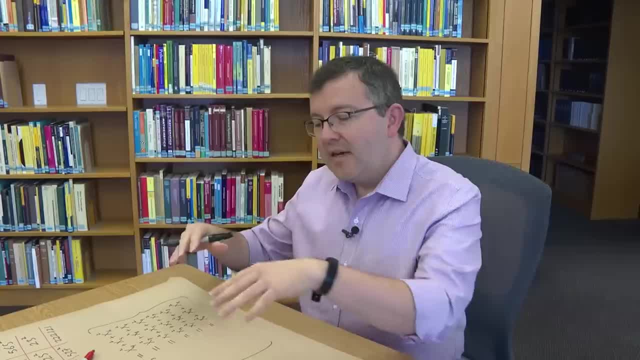 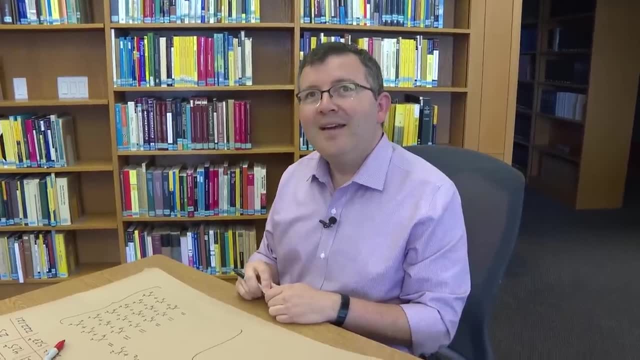 this particular system of equations, with the extra requirements that all these x's are different, And this is really sort of the important bit. I feel like you don't have to make that argument. to me It already looks difficult. but all right, Do you want more paper? 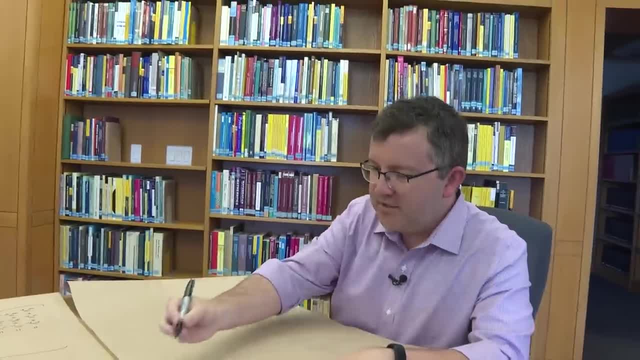 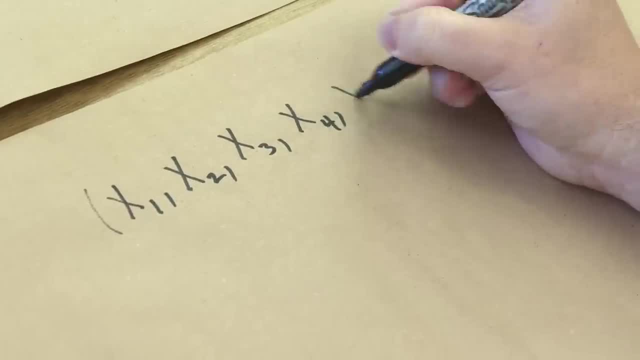 Sounds good. Yes, We have nine variables and we have these six equations, And so I want to think of these nine variables as like a point in some kind of space, And this space has to have room for this many coordinates. OK, So I want this to be a point. 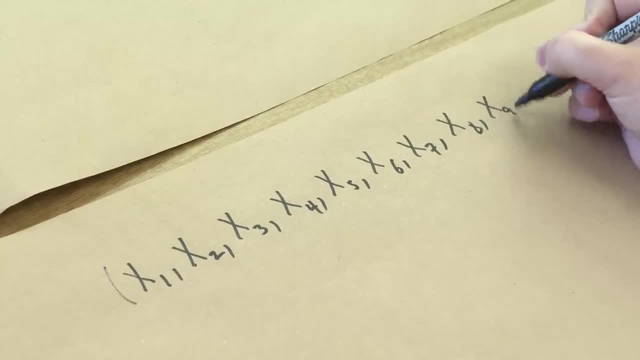 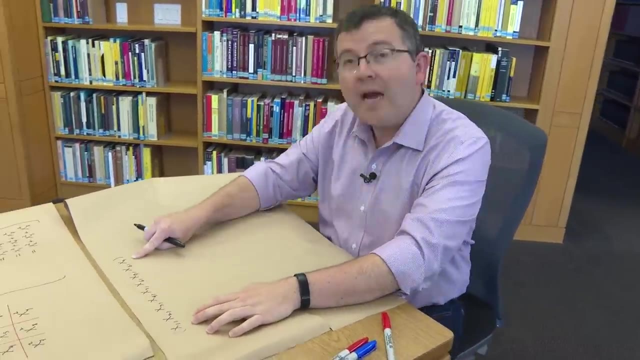 It looks like this is going to be a point in some kind of nine-dimensional space. you know Like usually we have like a three-dimensional space that has like x, y and z coordinates. There's only three coordinates Here. I'm going to need a space where I can write down nine coordinates. 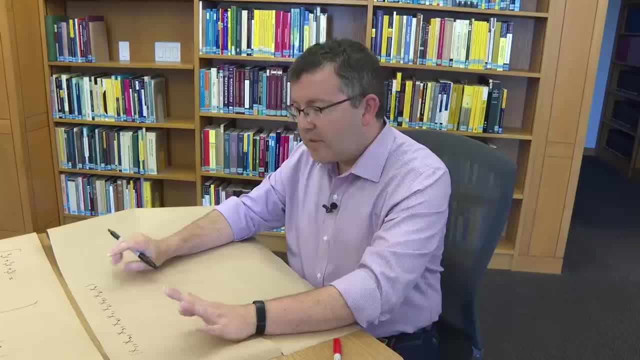 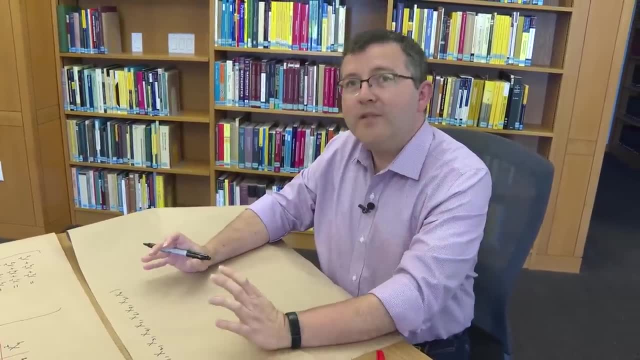 OK, So that looks like it could be a nine-dimensional space, But there's something really special about the equations that we have that allow me to cut things down sort of by one dimension Instead of sort of, even though I'm going to write my points using nine coordinates. 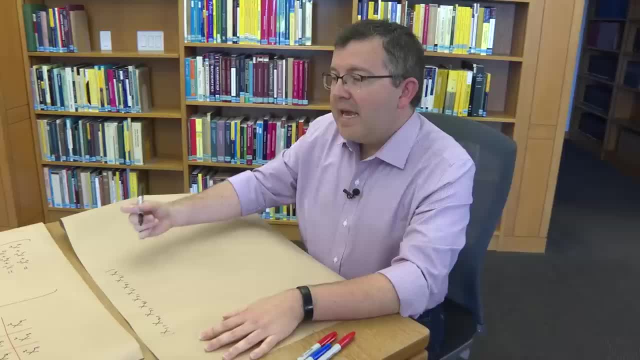 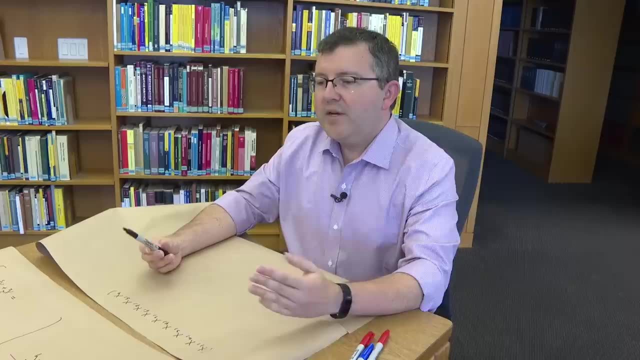 they're really sort of only eight dimensions that are in the works In the same way that we talked about. you know, some squares feel like you know they might be a little fake. There is a sense in which some squares, even though they appear different, they feel like 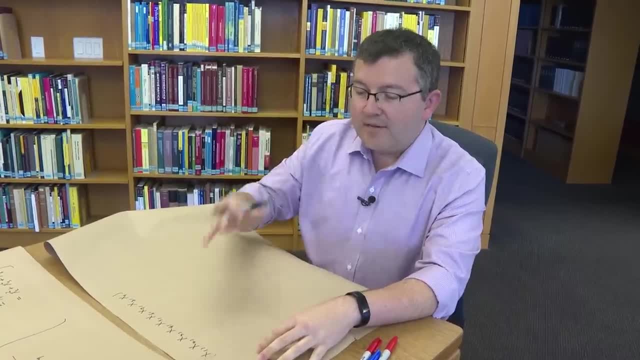 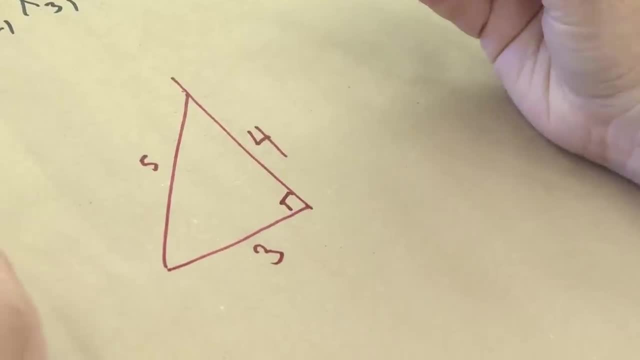 in our bones. they're kind of the same. OK, And let me kind of show you that with something that's probably a little more familiar, which is sort of the Pythagorean triangles. This is a very famous triangle, the 3-4-5 triangle. 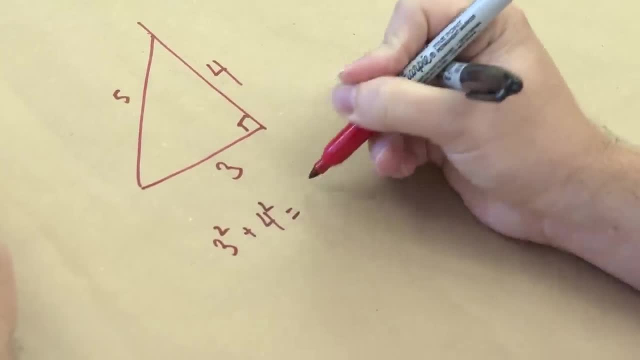 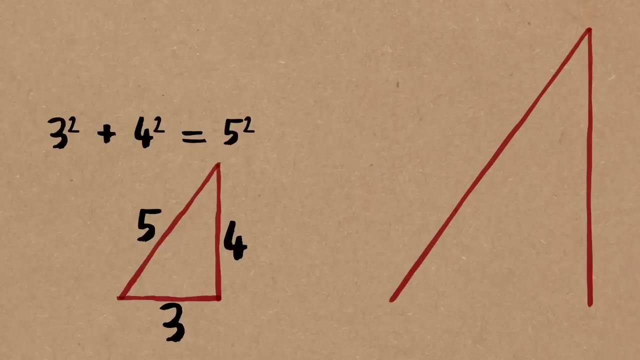 And we have that 3 squared plus 4 squared is equal to 5 squared. This is the Pythagorean relation. But you know, here's a. it's a different triangle, but this is going to be a 6-8-10 triangle. 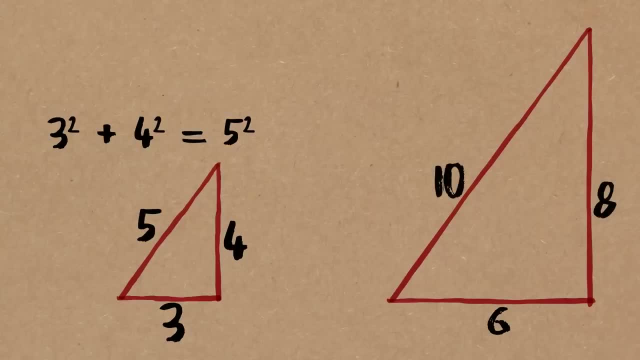 And there's something funny about this, which is that, OK, it's still true. So 6 squared plus 8 squared is equal to 10 squared, But somehow these triangles don't really feel that different. It just feels like I took this triangle and I just kind of scaled it up. 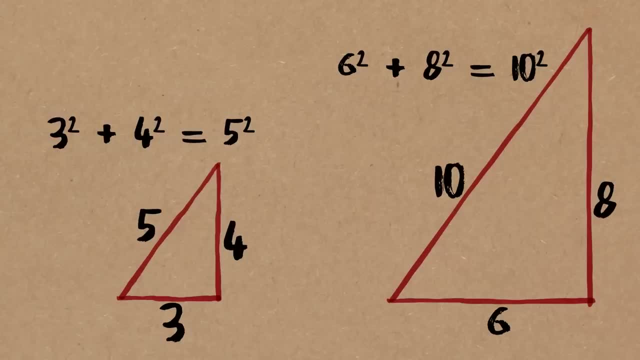 In a sense the you know, I don't know. You know the triangles literally are different, but they don't feel like a genuinely different triangle. It looks like I just took the triangle I already knew and I scaled it up. 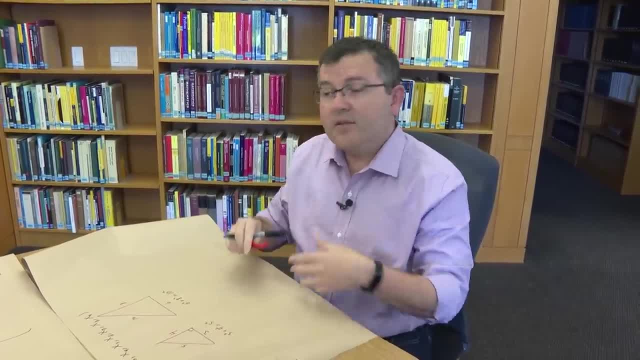 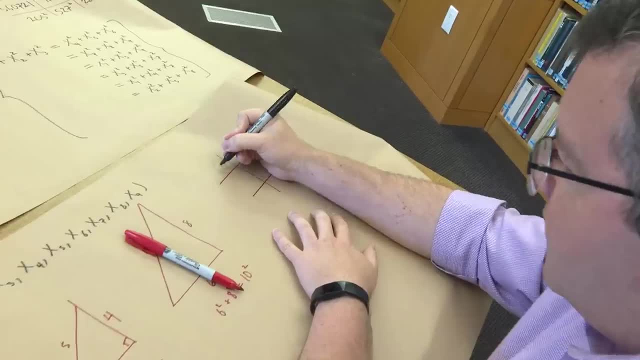 And the same thing is going to happen with things like magic squares. It doesn't even have to be magic squares of squares, right? There's a little shoe, And so I can just take the little shoe and just multiply everything by 2.. 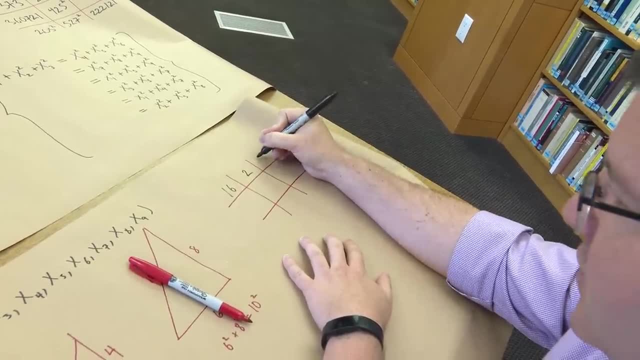 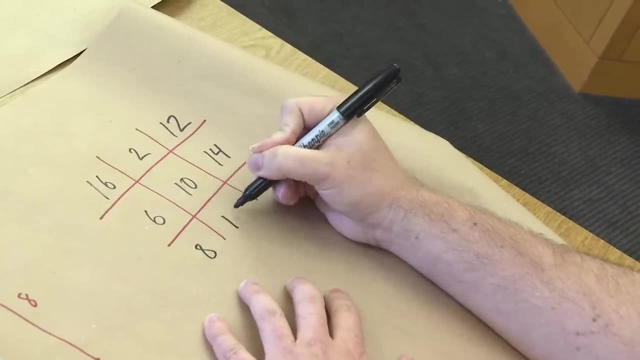 So I'm going to put a 16 here and a 2 there and a 12 there and a 6 and a 10 and a 14 and an 8 and an 18 and a 4.. OK, And now everything adds up to 30, this time. 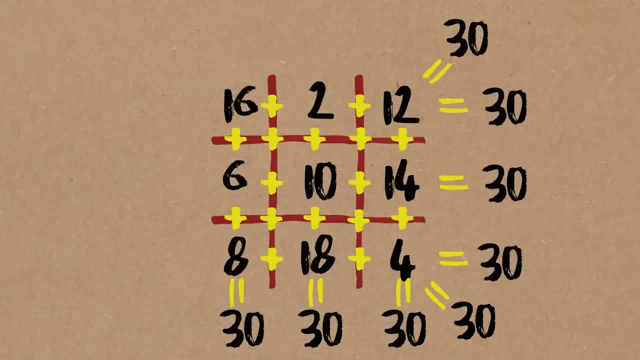 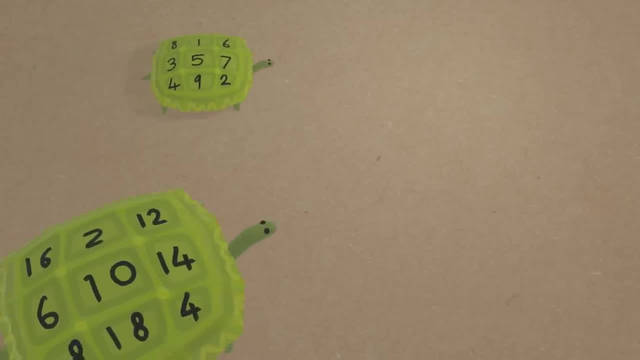 But that's not very surprising. I just scaled every single number by 2. And so you know the equations that give you a magic square. you know it's just like multiplying those equations by 2. And so this doesn't really feel like a genuinely different magic square from the low shoe. 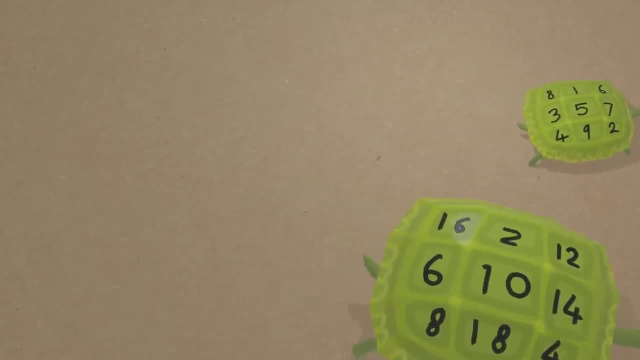 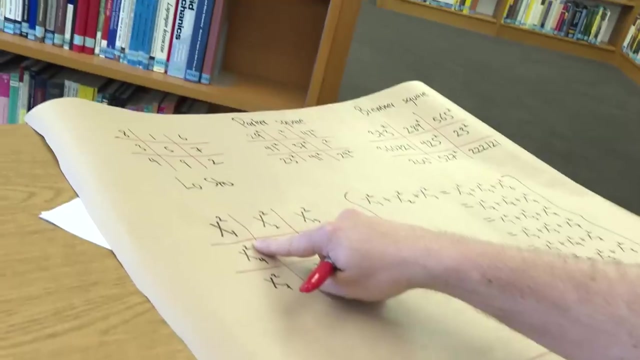 In a literal sense it is different, but somehow it sort of came from the same mold, And so that's really. the important thing is that when we look at all of these coordinates, and I multiply them by 7.. When I look at my magic square of squares, 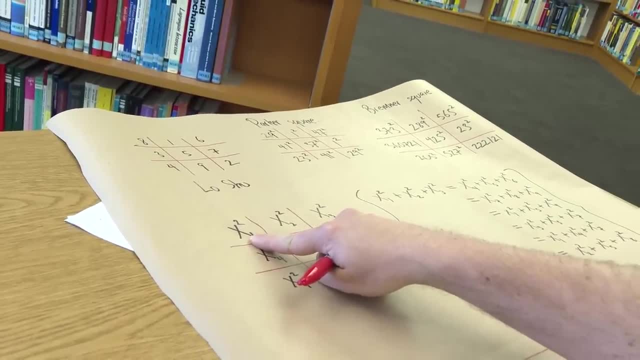 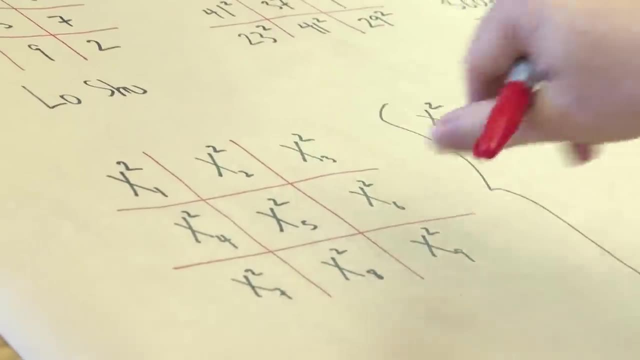 Each one of these entries will get multiplied by 49, because 7 squared is 49. And so every single entry will get multiplied by 49. And then it'll still be true that the rows and the columns and the two diagonals will add up to the same. 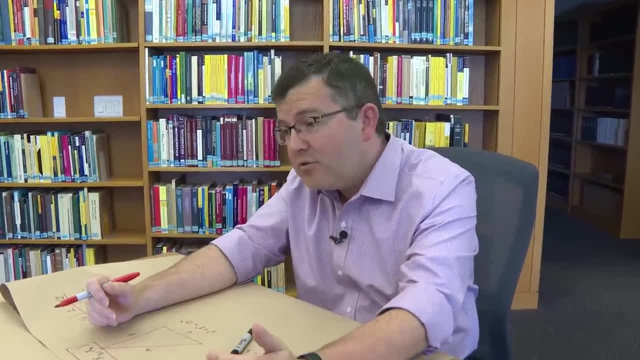 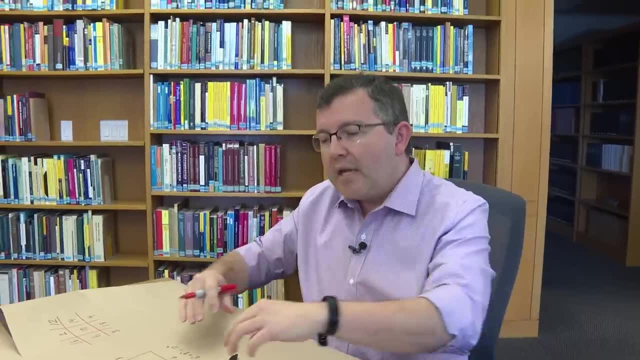 Any solution to this problem and I scale it up or down. I could also just have fractions instead in there I'll still have a magic square of squares. So these solutions have this very nice scaling property, And what that means is that even though you see sort of 9 coordinates, you only really 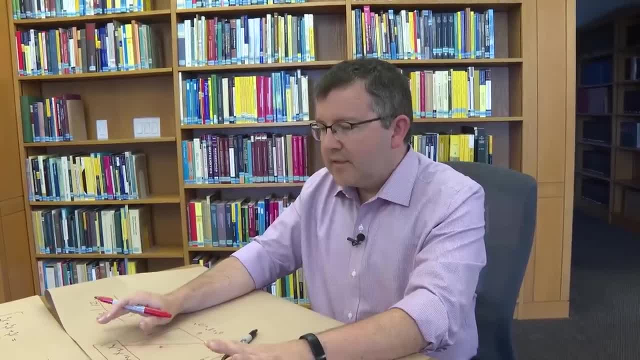 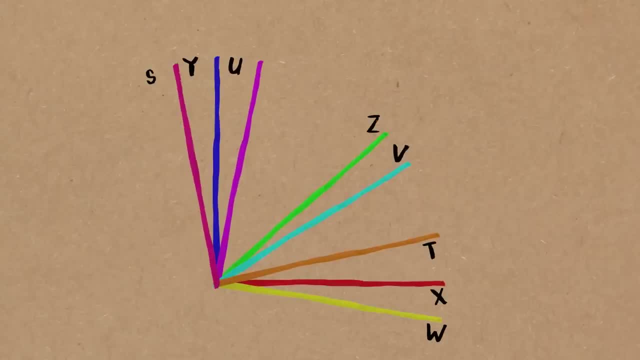 have about 8 degrees of freedom. So the reason that's important is that. So the natural habitat for these equations is something like an eight dimensional space. What do I mean by the habitat of an equation? So let me just remind you, you know, if I, if I just worked in the usual plane where 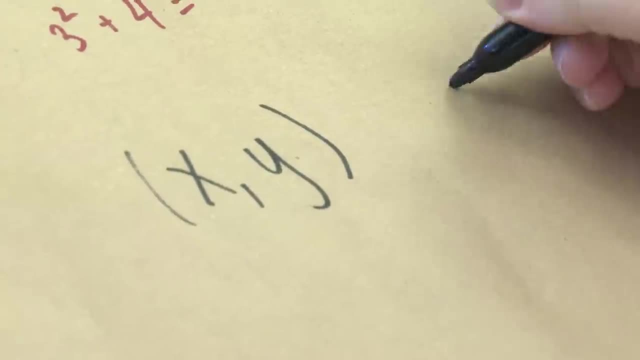 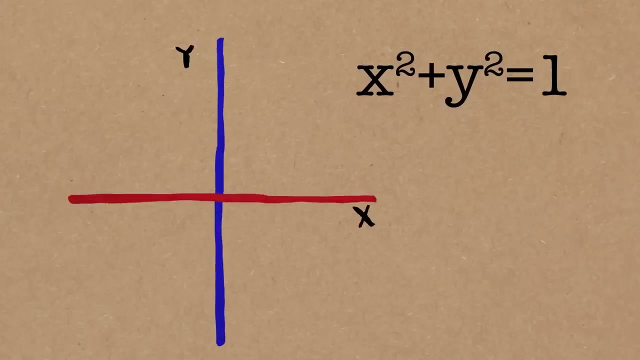 I had X and Y coordinates, so I had two coordinates. I have two dimensions. you know, I can look at an equation like this: X squared plus Y squared equals one. This is one equation in this two dimensional space and it cuts out for us a circle of 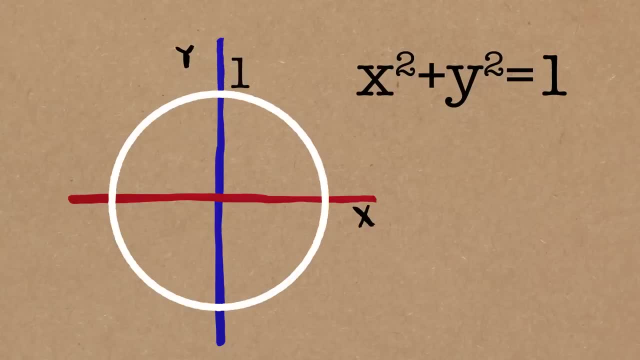 radius one. X squared plus Y squared equals one, And so what we're going to do here is we're going to do this. So what we're doing here is something similar. It's just much harder to visualize because I'm going to work in a space that technically. 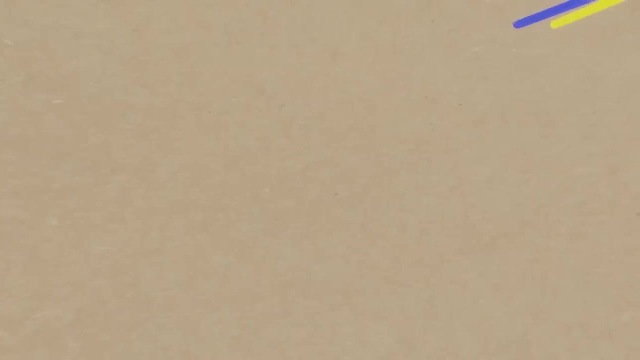 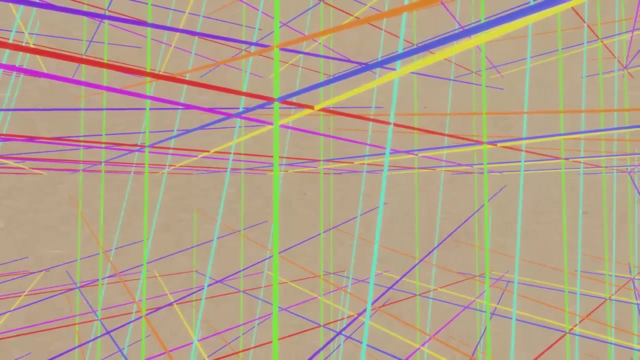 has nine coordinates but only really eight degrees of freedom. And inside that space I'm going to look at the solutions of some big set of polynomials, And this set of polynomials will carve out a geometric shape, just like X squared plus. 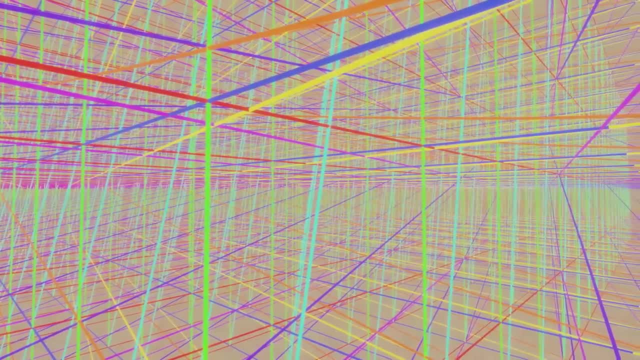 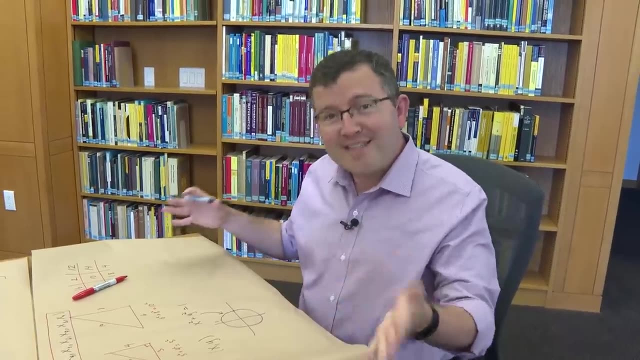 Y squared equals, one carves out a geometric shape on the plane. It's just that it's. you know, it's hard to visualize eight dimensional space, So I don't know how to draw that here. But the object is out there and it exists. 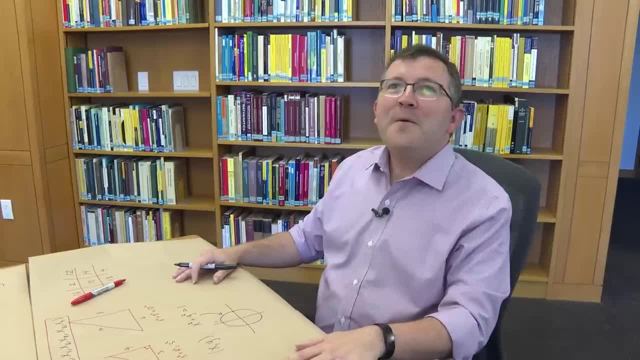 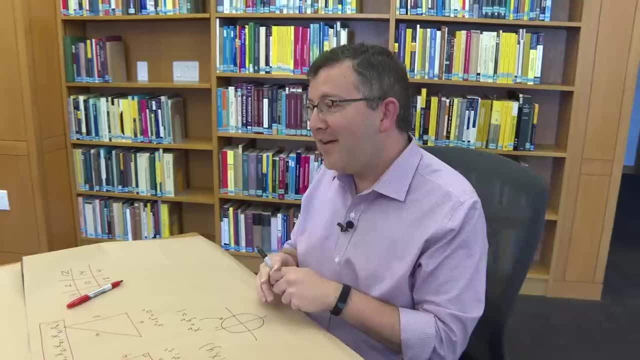 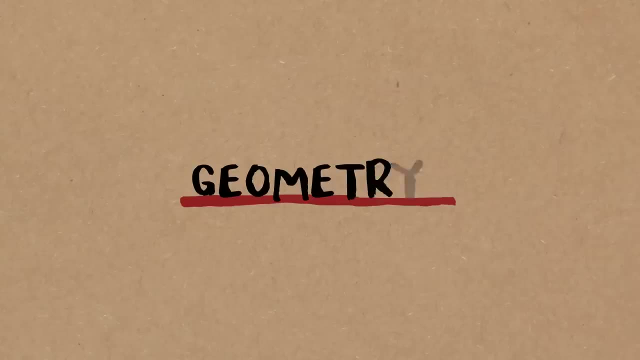 So not only is it impossible to imagine the playing field, you also don't even know what the configuration of the players are. Right, That's right, Yes, Yes. So we really have to sort of use our imagination and the algebra. This is sort of a really important idea that we're sort of trying to do some geometry. 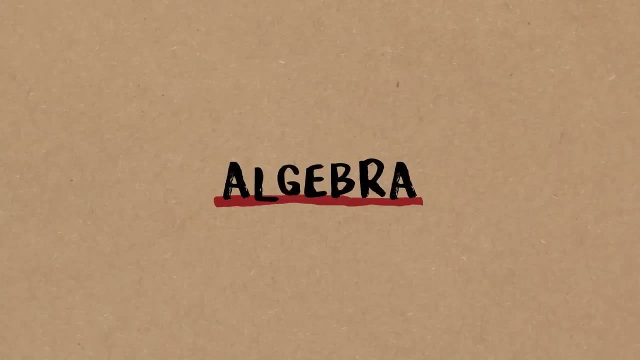 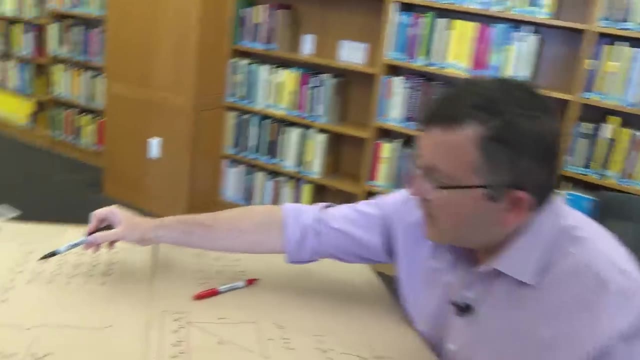 but when we can't visualize things, sometimes the algebra is still there and we can work with the algebra instead of the geometry. So we have this eight dimensional space, Okay, And if you look back at the set of equations that we wrote, there are six equal signs. 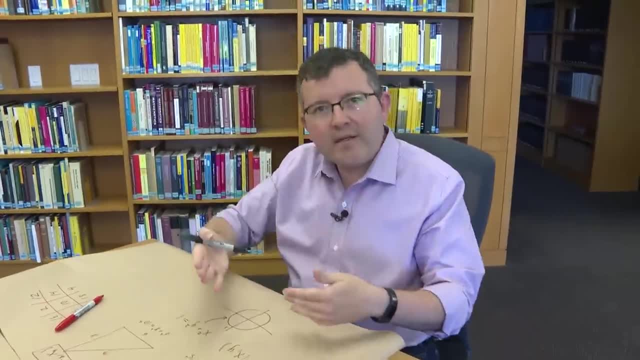 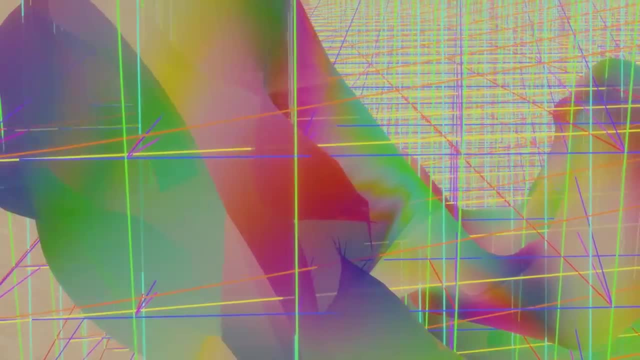 And so each one of these equal signs is putting a constraint on this eight dimensional space. So you start with this eight dimensional space, and then I put a constraint in it, And so now what I'm holding is probably a seven dimensional thing, And then I put another constraint in it. 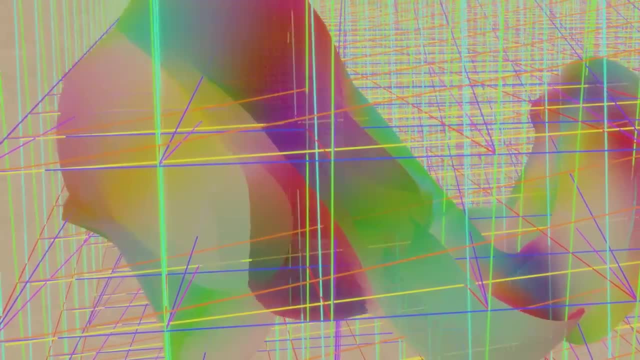 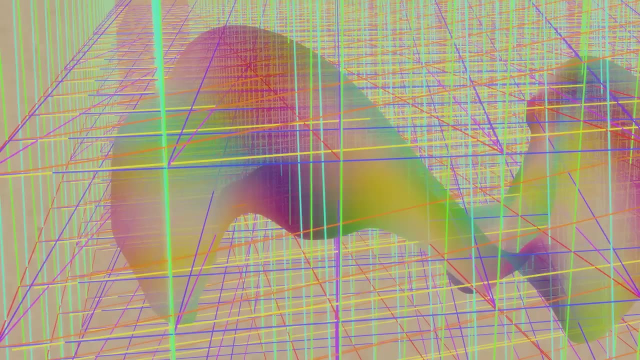 And so now these two constraints have to be satisfied simultaneously, And so the intersection is probably something that's six dimensional, and I keep doing this, And if I have six constraints, well okay, I'm just, you know right, Eight minus six. 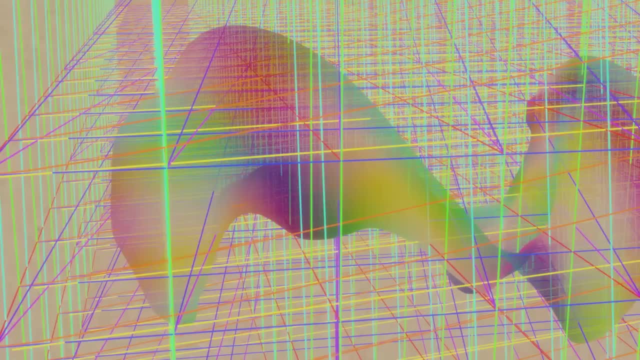 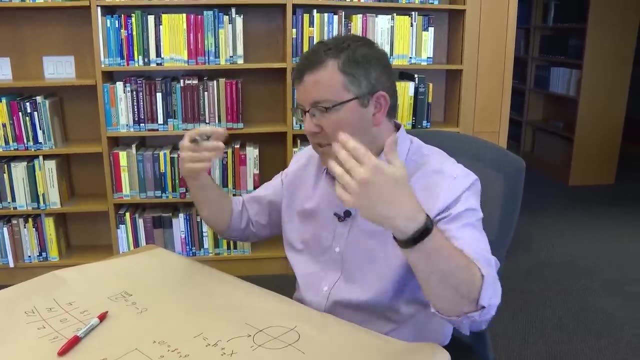 Six is equal to two. Once I sort of put all these constraints together, it looks like what I should have is some kind of surface, some kind of two dimensional thing. Each constraint is sort of cutting me down in one dimension. I started with eight degrees of freedom and I've taken away six. 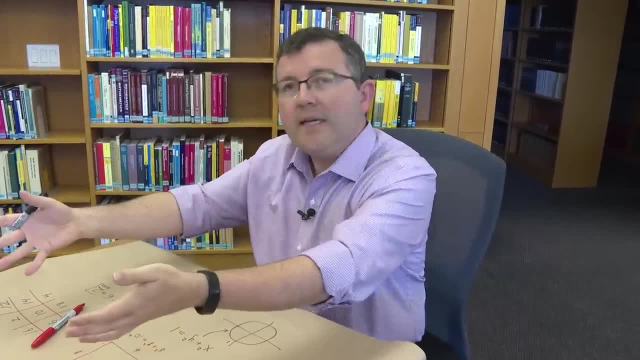 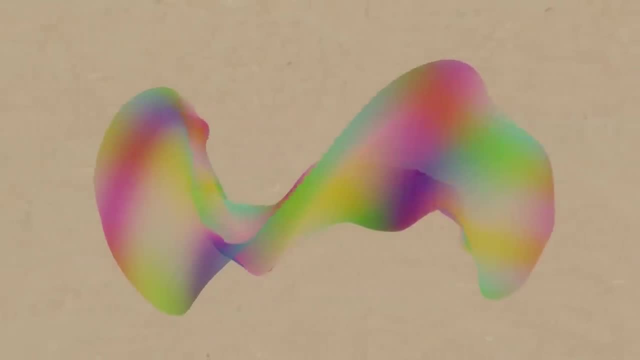 And so, even though it's very hard to actually visualize something like this, it looks like it could be some kind of surface, So there's some two dimensional surface that would hold the key to everything Exactly. This is exactly the point There is out there. 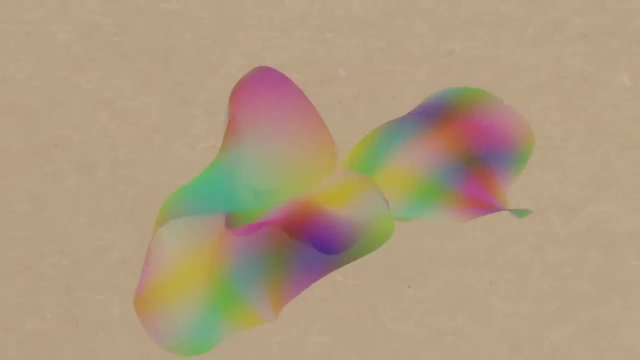 There is this sort of incredible you know. now I'll just do like a metaphor for it. There's this two dimensional surface, and each point on that surface is going to have coordinates: X one, X two, all the way to X nine. 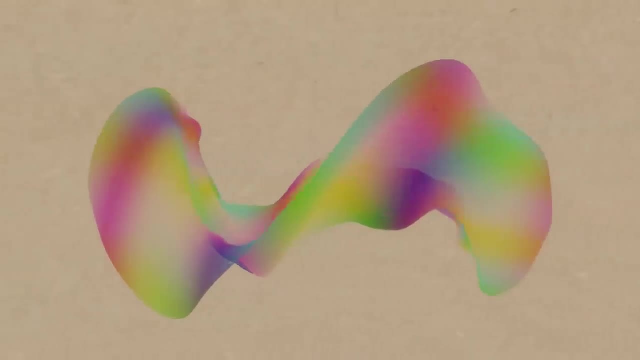 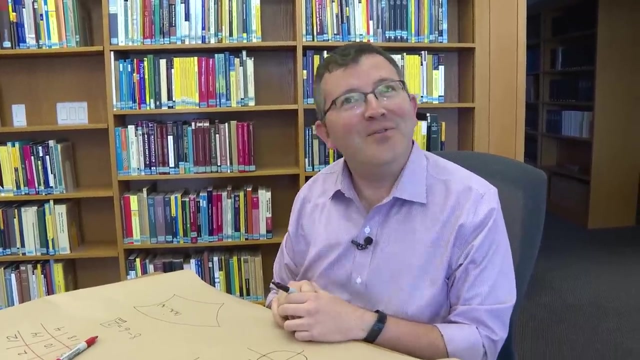 And this point encodes one of these magic squares of squares. Now, what's important, Has this surface got a name? Uh, I know, Can I suggest one? What would you like to call it? The Parker surface? That's awesome. 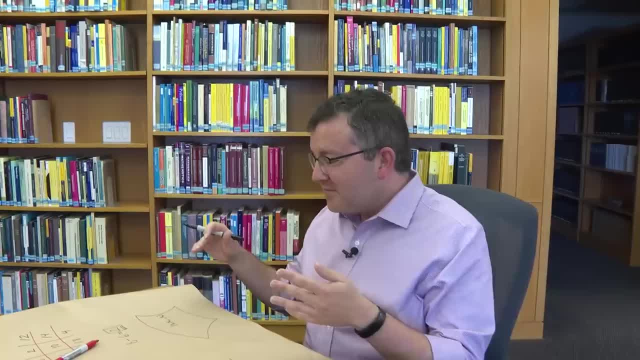 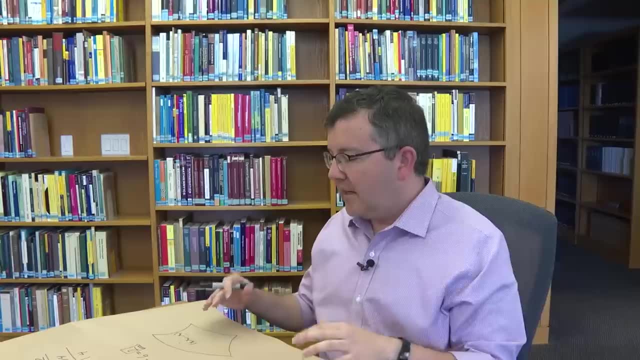 Okay, All right, Okay, Let's call it the Parker surface. Yeah, So so any point on the Parker surface is going to give you a magic square of squares. Now, this surface really is there. I think one of the things we have to realize is that that these X's could also be like 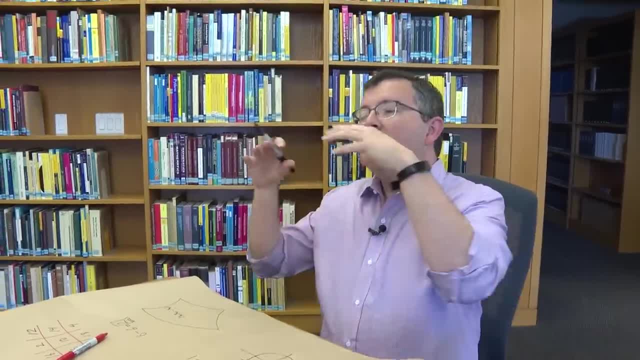 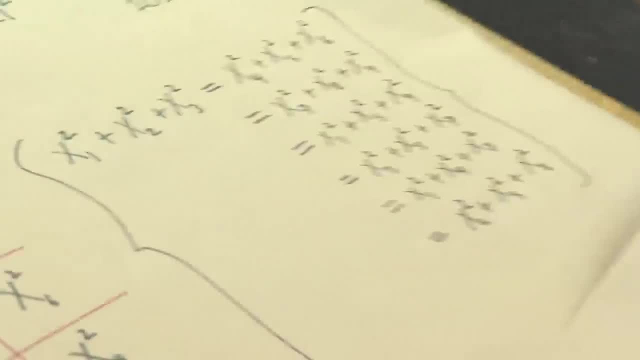 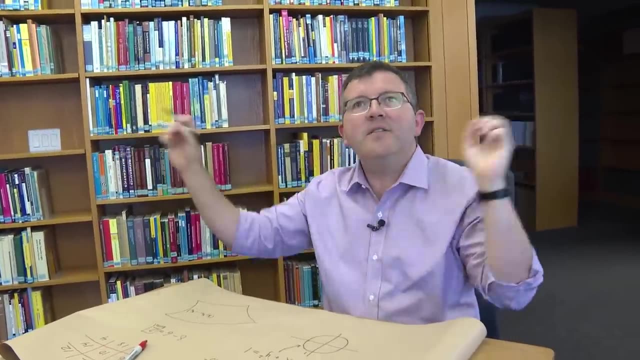 not just integers. right, We are looking for integers, We want integers, but but you know, if I just sort of write out these equations and I let X one through X nine, you know, be more general numbers Like pi or E or you know some something with an infinite decimal expansion, that's. 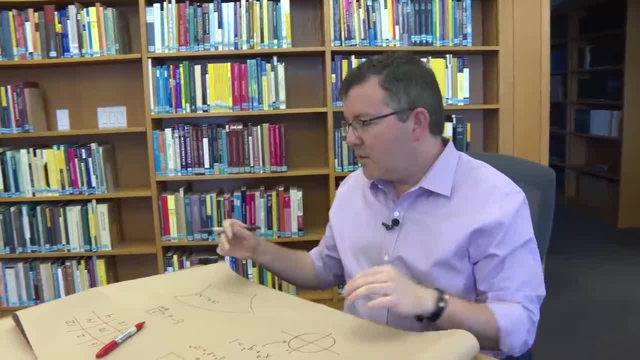 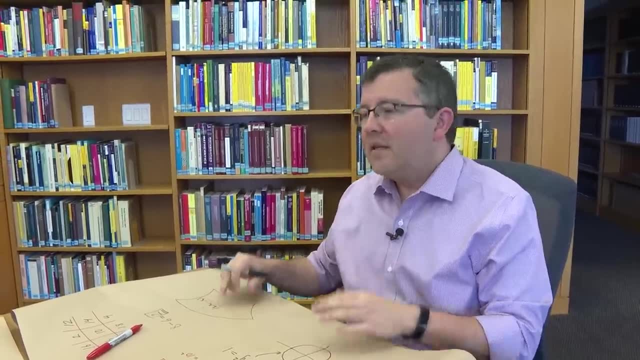 random. Um, those are perfectly good numbers too, And so what happens is that the square is there, but almost every time you write one of these points down on it, there's at least one coordinate. That's just not going to be an integer or a fraction. 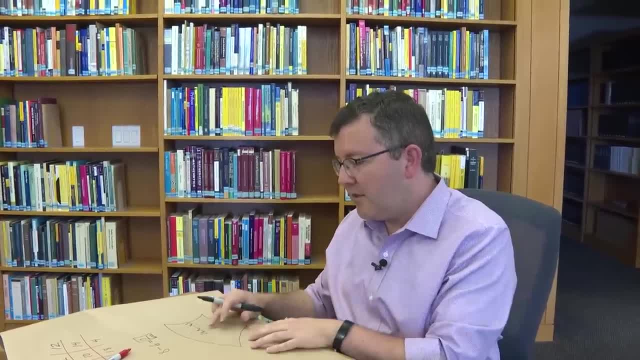 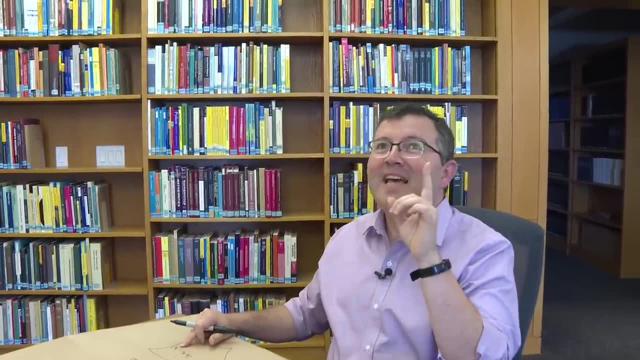 And so, so what we're really trying to do is, you know, our job is to try to find points on the surface all of whose coordinates are integers and distinct. Okay, And this is, this is where things get tricky, because inside this space, right, you can. 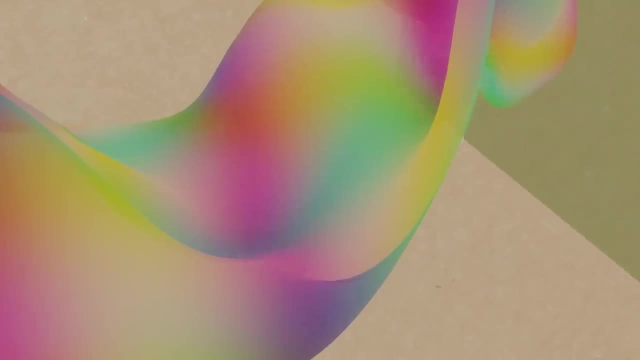 actually take something that looks kind of like a plane and then it'll sort of cut the surface and this will be, for example, the locus where, like, maybe two of the coordinates are the same. That could definitely happen. And you know, things like the Parker square, you know, have the property that some of the 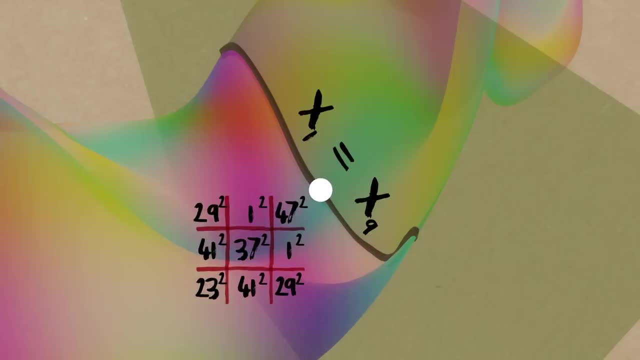 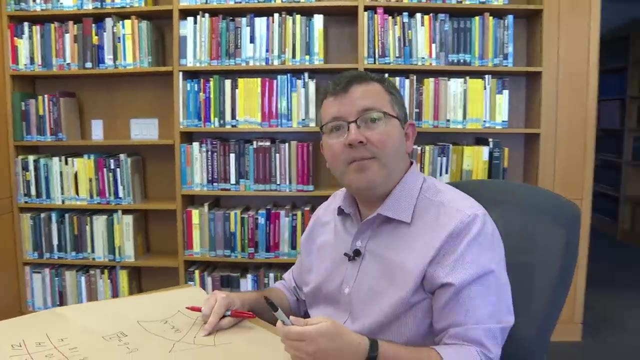 entries are the same And so, for example, it can be a point that happens to Lida. And this is the tragedy that we seem to face. is that, on the surface, every time we have a point, Yeah, You know, if we have a magic square of squares, these points tend to lie on these very special 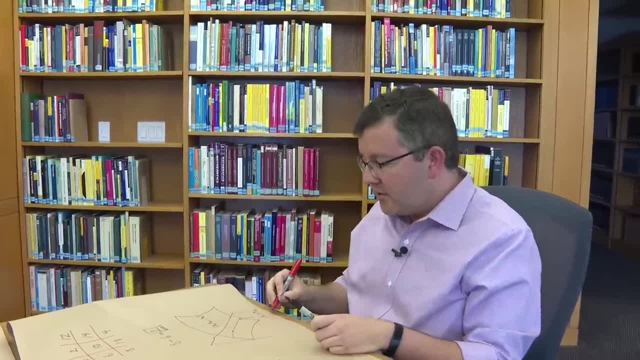 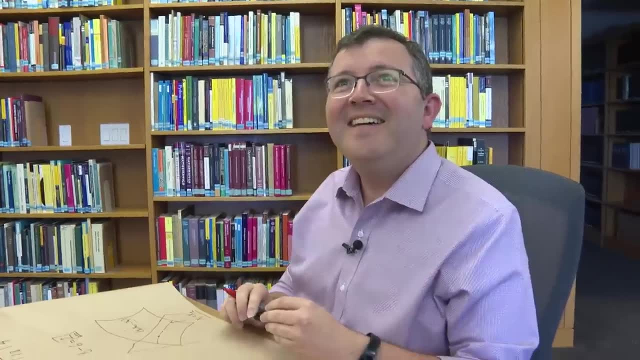 curves of the surface where you have conditions like you know, x1 is equal to x2, or x3 is equal to minus x7, or something like this, Because when you first told me about this surface, I thought maybe there'd be no points. 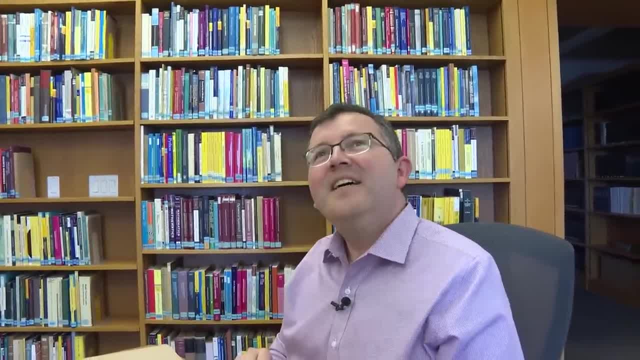 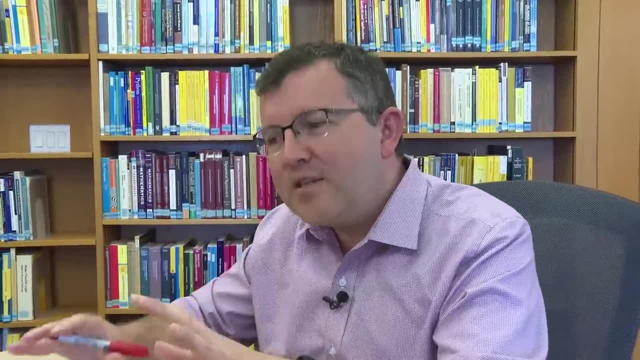 on the surface, where all, all of them are integers, but there are some there. so That's exactly right And- and this you- you hit on something really important, Brady, which is that this is what makes this problem really difficult. 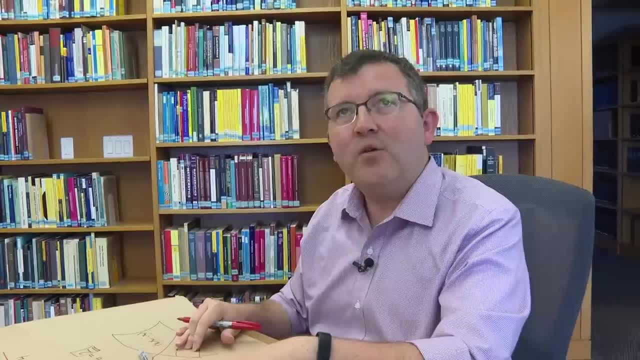 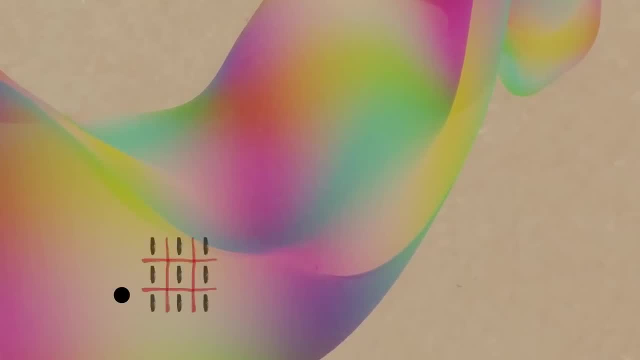 Is that that this surface really has points with integer coordinates. It's just that we don't like the points that we see. There's also the one where you set everything equal. just put everything equal to one. That's a perfectly good point on the surface. 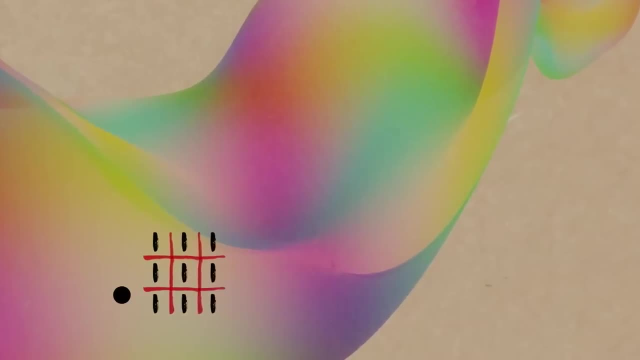 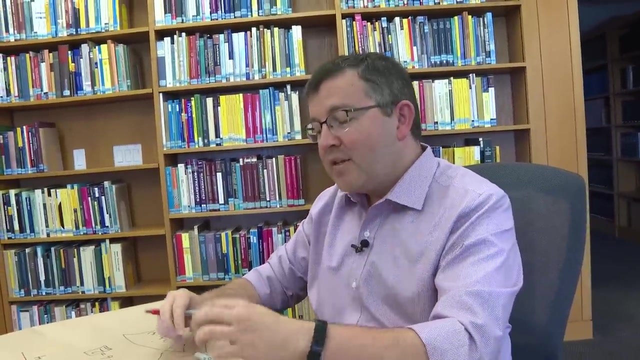 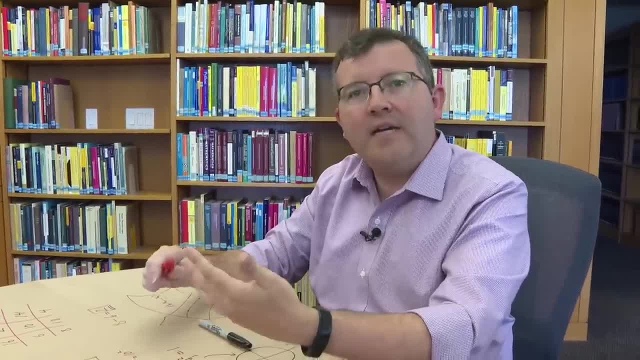 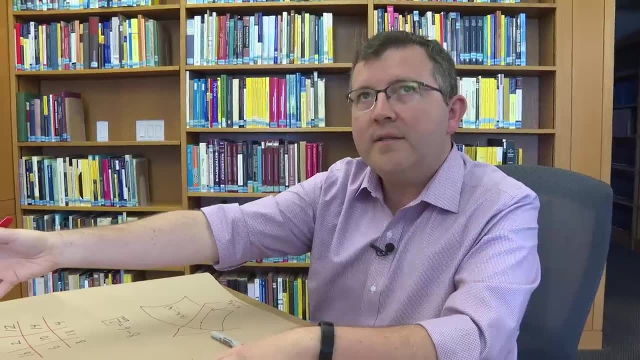 Yeah, So, and this is what makes it hard. So, so in in there's this area of math called Diophantine geometry, that that tries to exactly solve this kind of problem, where you take a collection of polynomial equations, like the ones that define the magic square of squares, and and they try to find integer solutions. 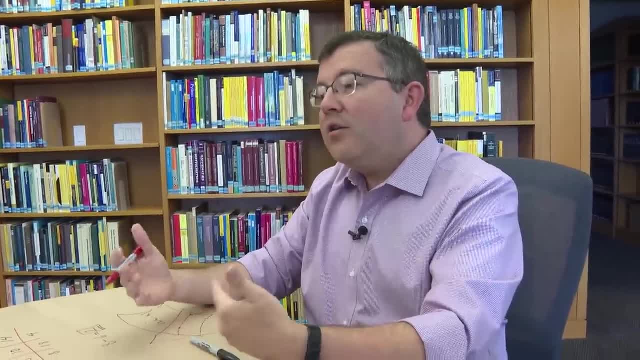 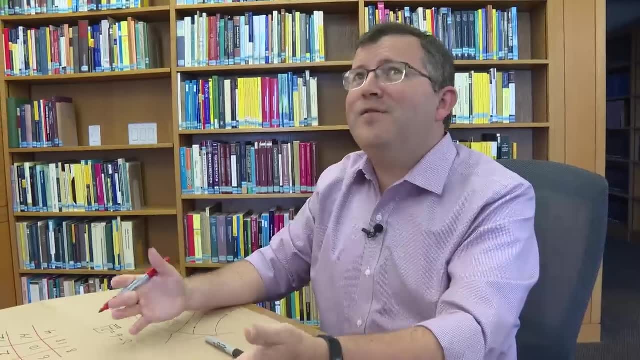 or prove that there are no integer solutions other than sort of you know, a few obvious ones that we see but that we're not really interested in. The same thing happens with Fermat's Last Theorem, which is really aggravating. 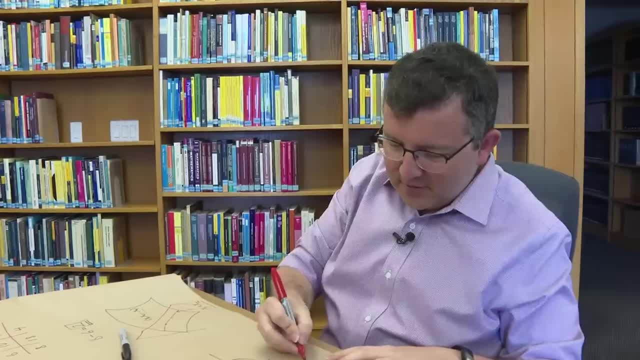 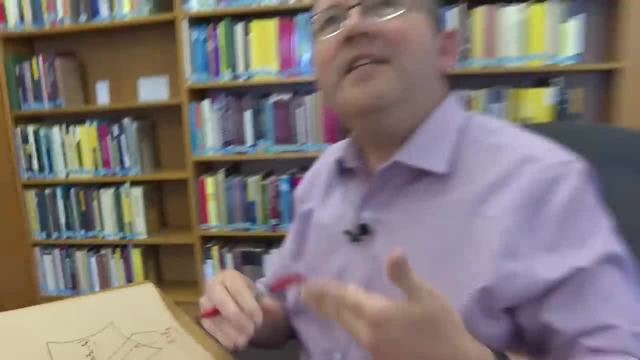 You know, Fermat's Last Theorem has solutions, right? You know, zero to the n plus one to the n equals one to the n. So the Fermat equation has solutions. What makes it really difficult is to show that there are no solutions other than you. 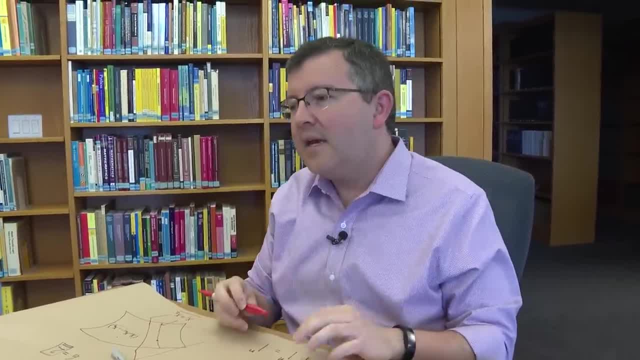 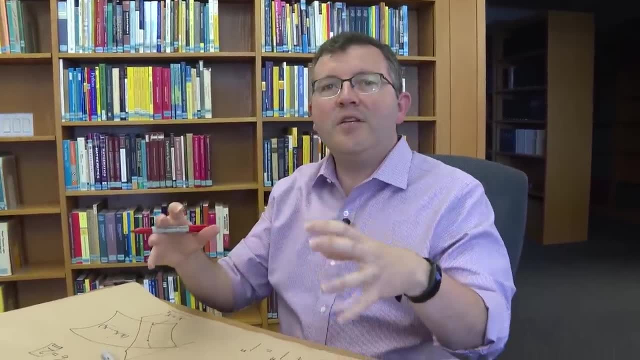 know the solutions that contain at least one zero. Okay, And that's. that's a much more difficult problem. In math we have all these. you know this whole slew of techniques for showing that systems of equations have no integer solutions whatsoever. 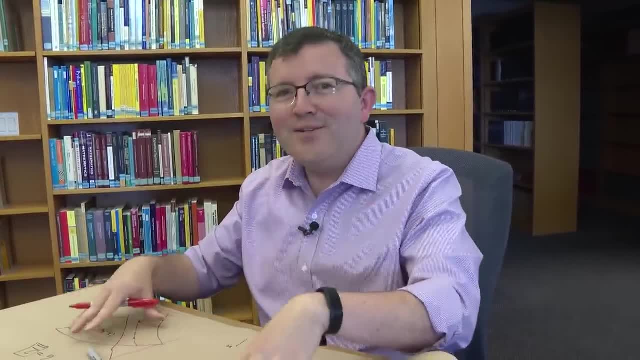 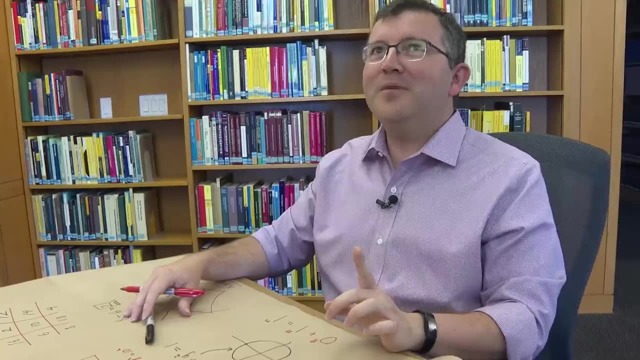 But that's not the case here. There are integer solutions, So what we're trying to do is to show that there aren't solutions other than the ones that we actually see, And that's a much more difficult problem to solve. You told me earlier that you've come to the conclusion that it's really unlikely that. 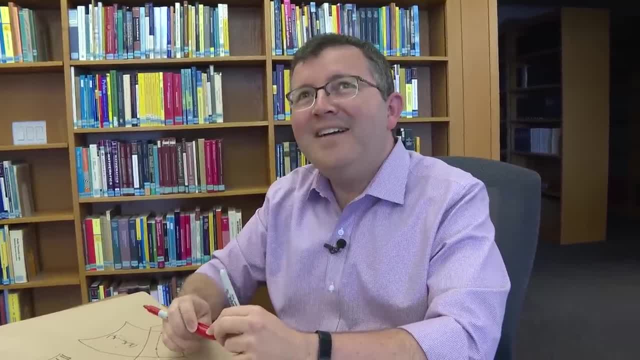 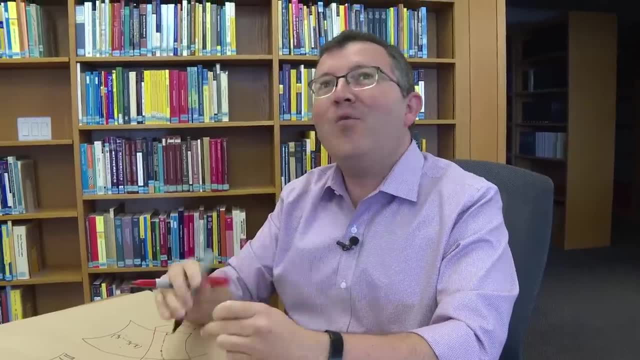 one of these exists. What you have shown me so far has made me more hopeful that one exists. Yes, I understand what you're saying. So why do I think that one might not exist? Okay, Yeah, I guess I yeah. 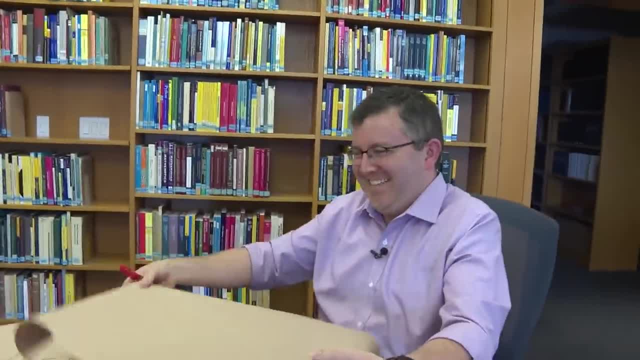 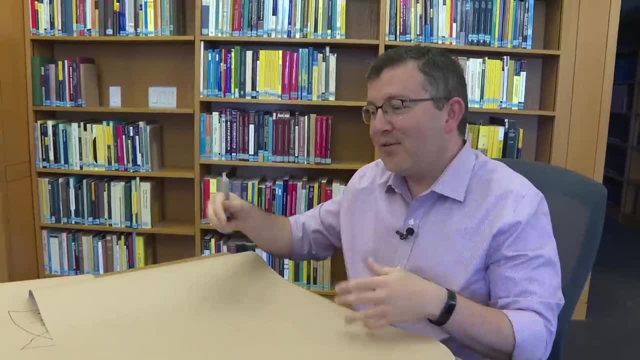 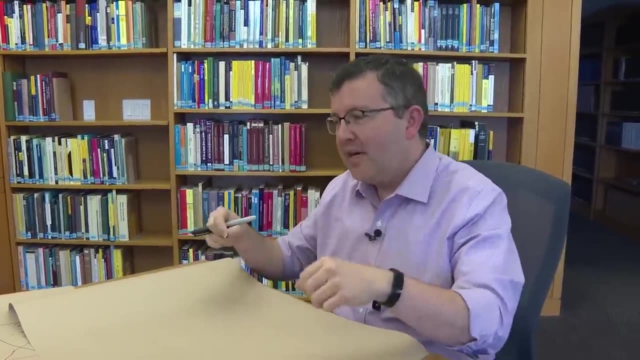 More paper. I need a new sheet of paper. Yeah, More paper. Take away my hope, Okay. So I'm going to try to explain why I think that, even though we have this huge surface worth of points, all of which actually give you a magic square of squares, there's just 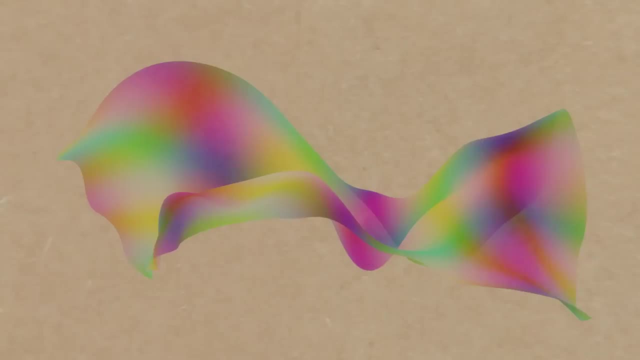 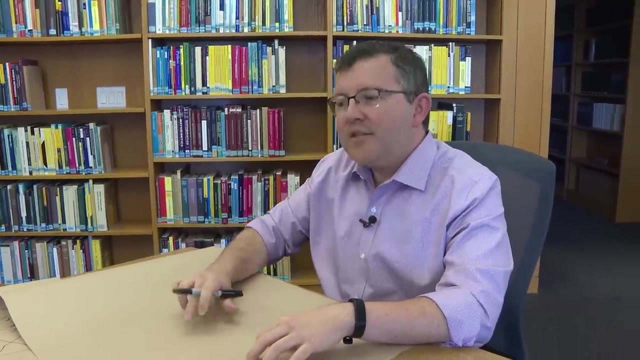 no point where all of the entries are integers and they're distinct. Why do these points even exist in the first place? And so this is a philosophical point, but it's you know. points that satisfy polynomial equations- that are, you know, all integers- are very, very rare. 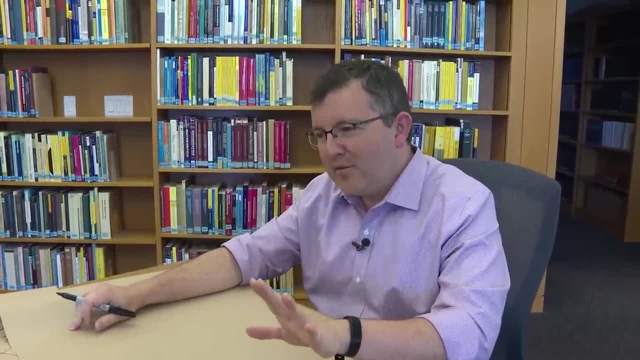 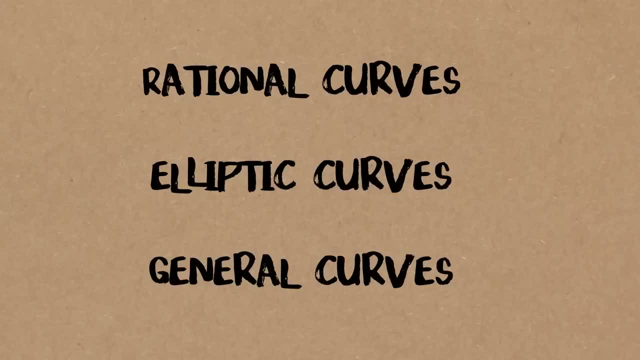 They're sort of almost accidents of nature, And this is sort of something really important to bear in mind. So we know if, instead of a surface, if we had a curve curves come in sort of three flavors from this sort of integer arithmetic point of view. 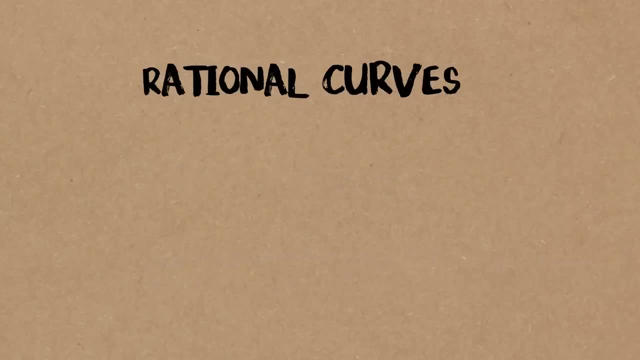 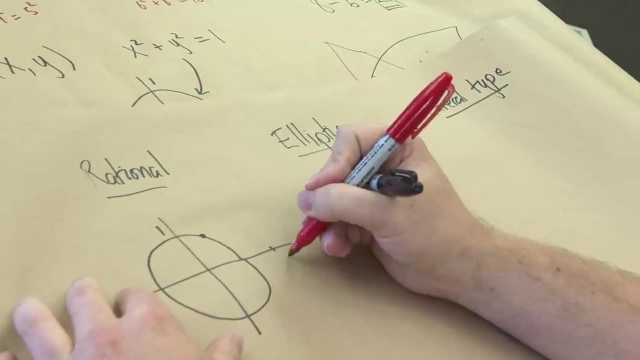 The first one is called rational, and in fact the circle that we were looking at before this is kind of a perfect example of a rational curve. what makes these curves themselves have lots and lots of points that have either rational or integer coordinates. 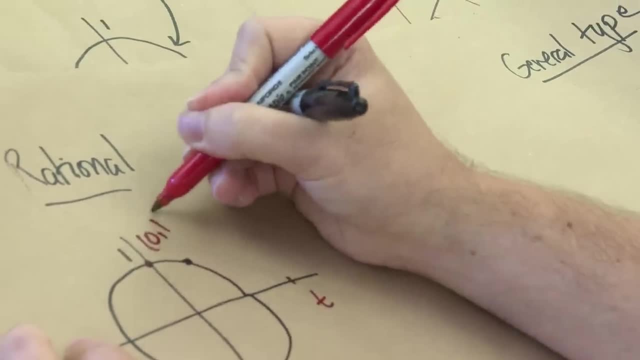 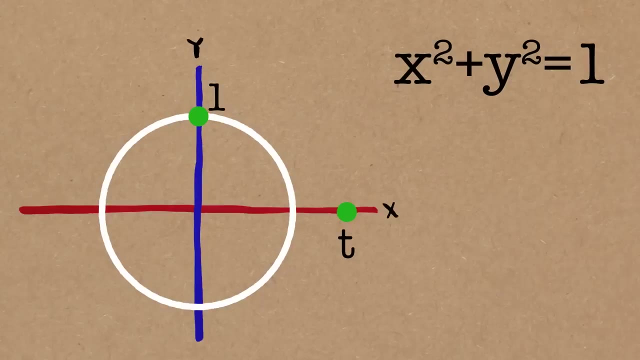 You know, here's already a point on the surface, zero one. If I sort of take the line Okay, This line that connects that point to some number t on the real number line, then I can do a little bit of analytic geometry and compute this thing. 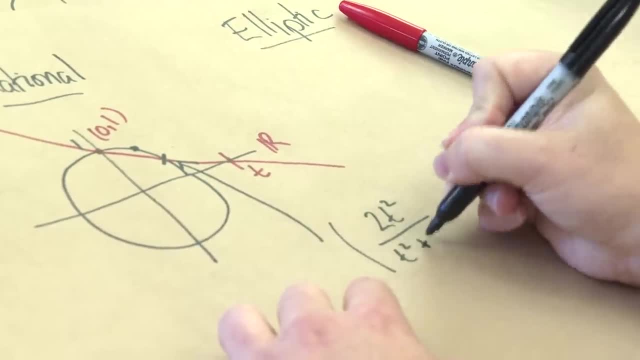 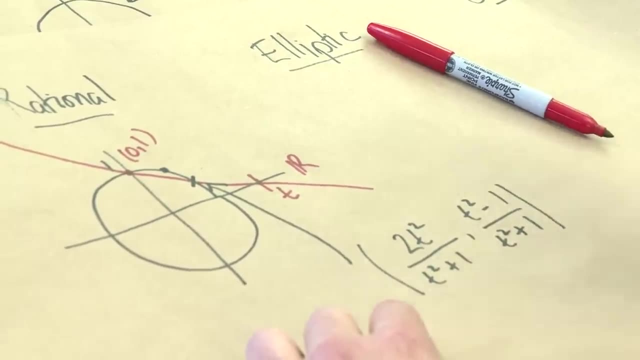 You'll see that it's two t squared divided by t squared plus one, and then t squared minus one over t squared plus one. This actually has to do with Pythagorean triples, but that's a story for a different day. What's important here, you see, is that if t is like an integer or some rational number, 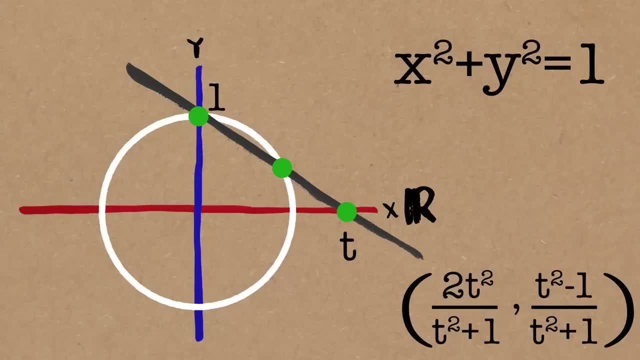 then these expressions are also going to be integers or fractions more generally. There's heaps of rational numbers on the real line, And so I just pick some rational number, t, and I do this construction, and it gives me a point on my curve that has a rational coordinate. 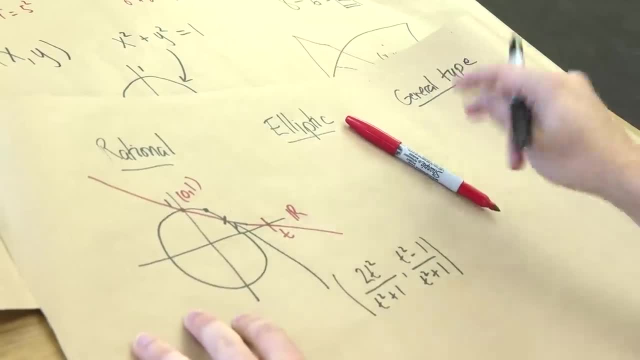 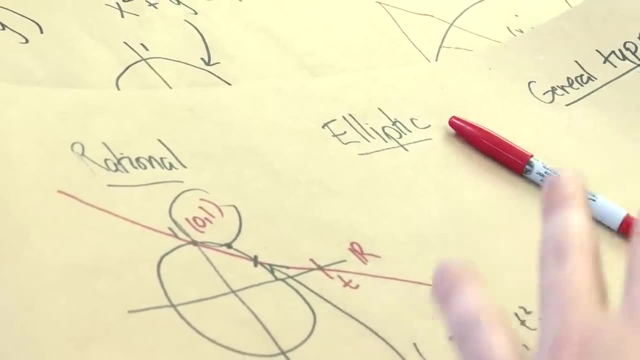 So rational curves have this like incredible property that the moment you have one point, okay, I need one point to get started. then I can use that one point to construct lots and lots and lots of other points. Then there's elliptic curves. 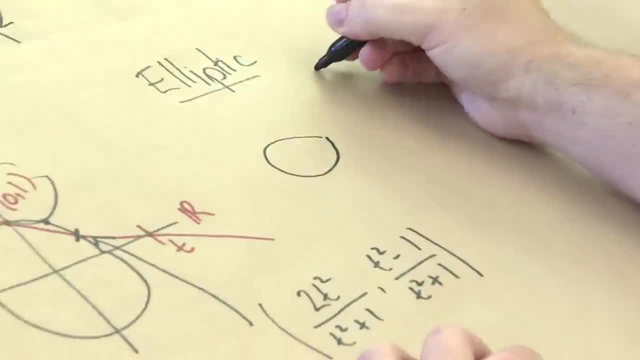 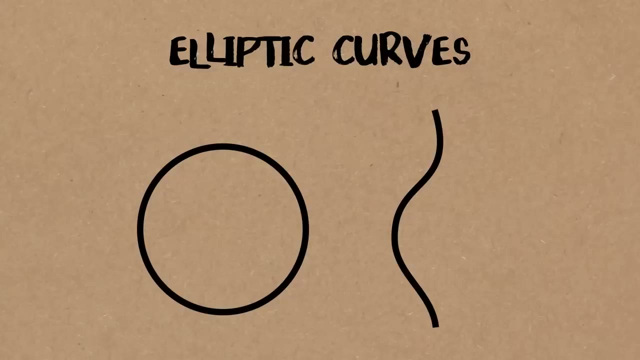 So elliptic curves sort of have this funny kind of shape. usually They're defined by cubic polynomials. Elliptic curves have this incredible thing That you can add points on them. Okay, So if I take p and q, okay, this is not p plus q, but if I just sort of reflect it down, 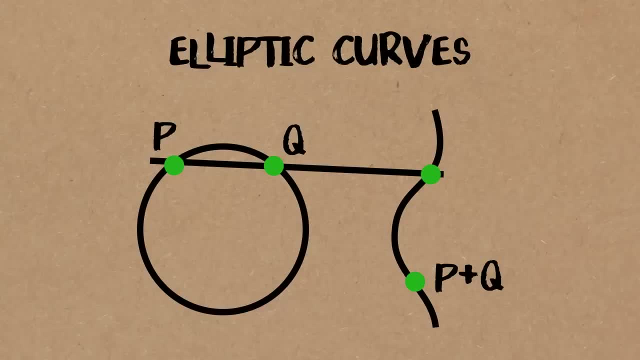 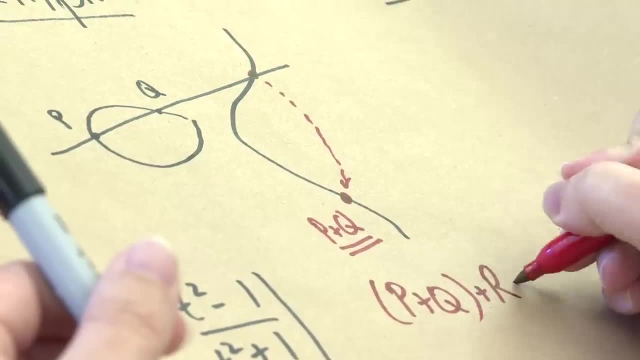 I can call this p plus q, And this sort of crazy little construction that I just did happens to actually sort of satisfy things like associativity, which is something that you know. if I have three things, you know, I can move the parentheses around. 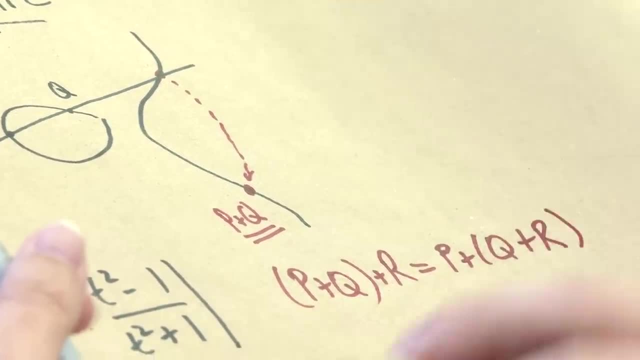 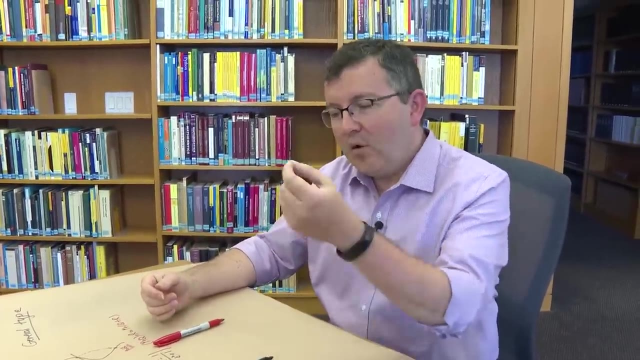 So elliptic curves have this crazy property that you can add points on them, And the reason that's important is because it allows you to also create new points out of old points. Okay, So if I have a new point, I can add it to itself, for example, and then create a new. 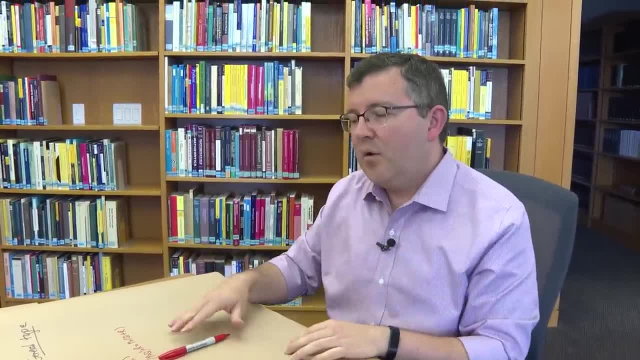 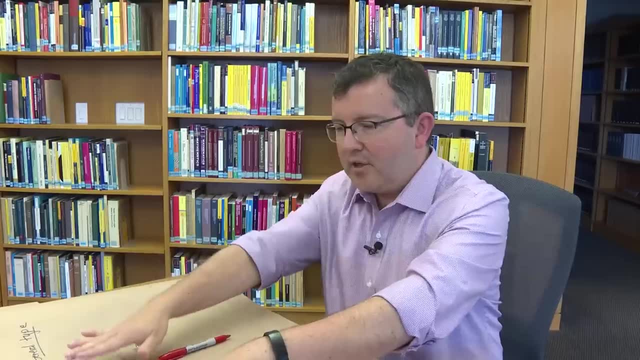 point, And then I can add that point to itself and create a new point. And so elliptic curves have this, also this property that if I start with a point I can propagate it. So rational curves are great. Elliptic curves are great in that, you know, they can come with lots of points. 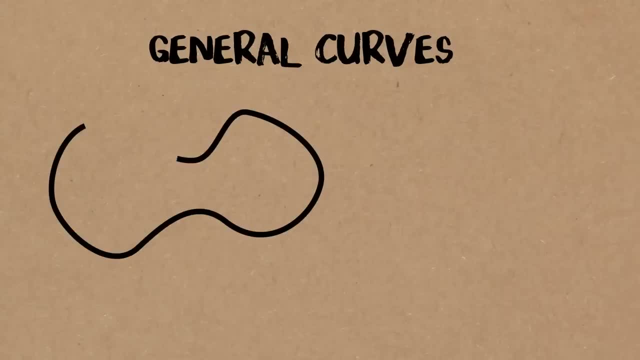 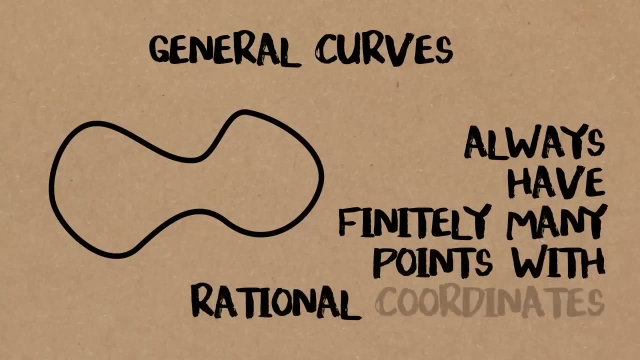 And then there's general type curves And those are sort of well. they're sort of more complicated, But one thing that's amazing is that they always have finitely many points with coordinates that are rational. This is a spectacular theorem. 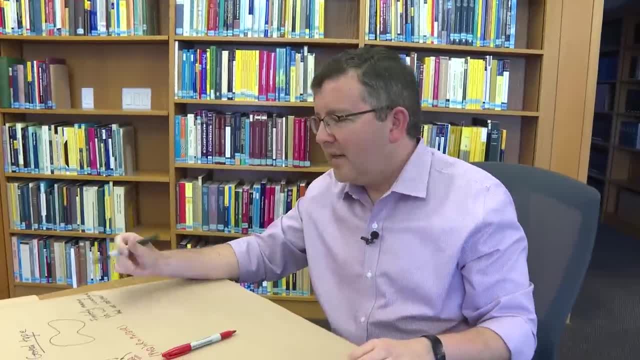 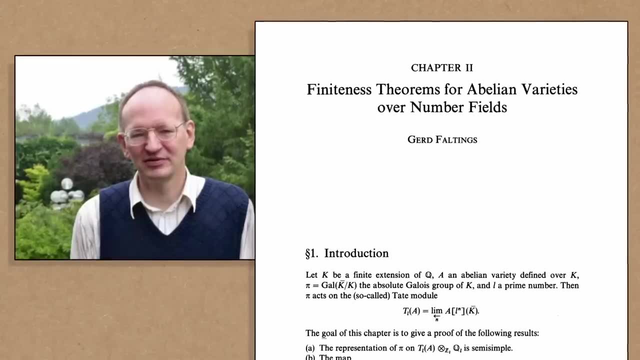 Okay, It's called the early 80s, maybe 1982. It was proved by Faltings And he got the field medal for this theorem, So this was sort of a big, big deal. It was called the Mordell conjecture back then. 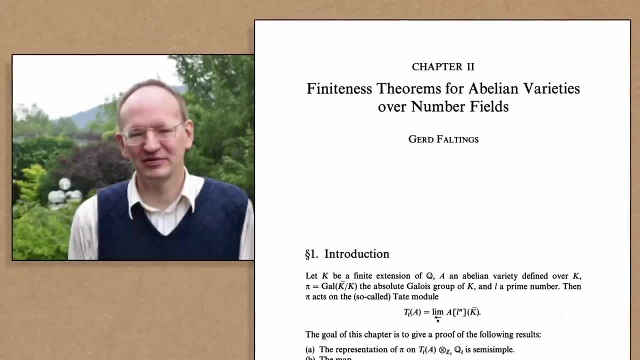 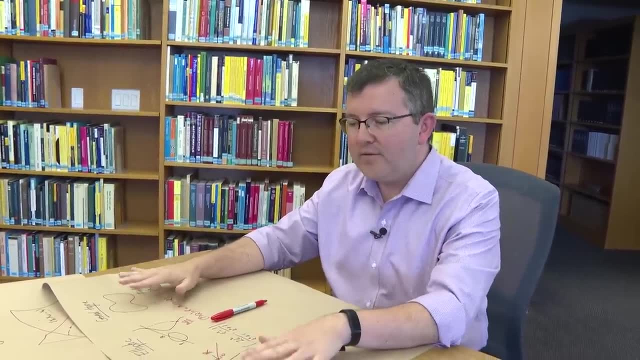 And now it's Faltings theorem: What we have is not a curve, Okay, It is a surface, But I'm telling you this story because it actually plays a very key role in our surface. So when we have curves, they sort of come in three different flavors. 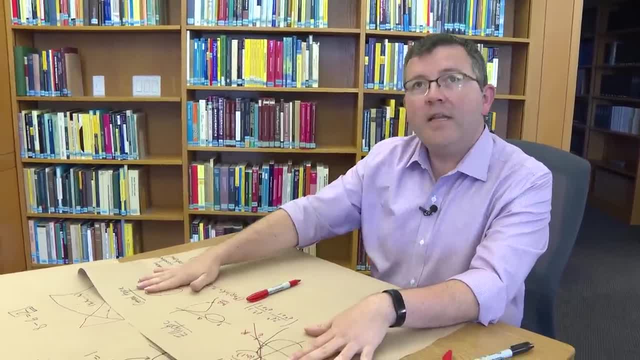 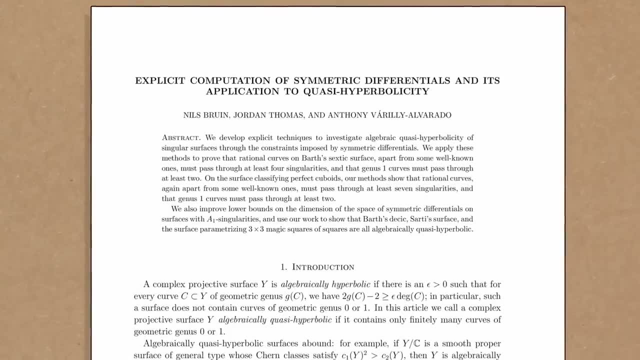 Two of those flavors have lots and lots of points And one flavor does not. So what happens with the surface that we were calling the surface, The Parker surface, right? Is that, as a consequence of some work that me and a couple of coauthors, Nels Brown and 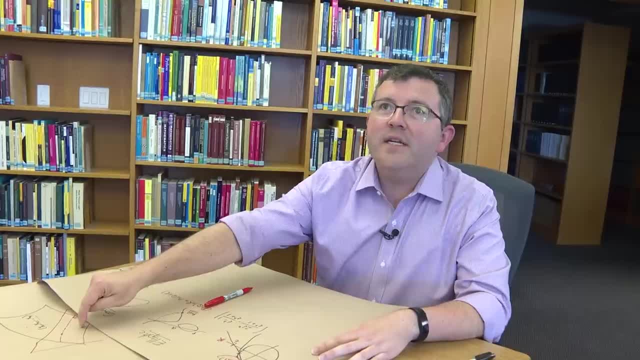 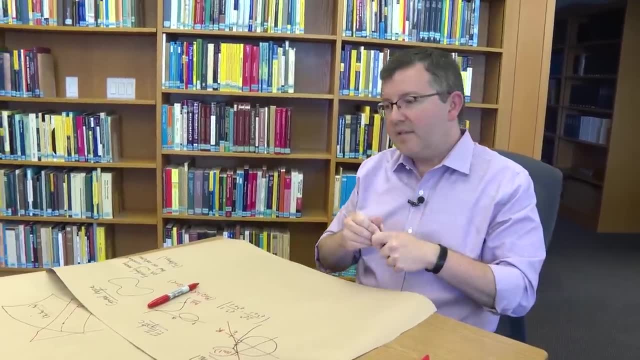 Jordan Thomas were working on is we managed to show that on this surface right here, there are only finitely many curves of these two types, And this is really something that surprised us. So a surface is full of curves made of curves. 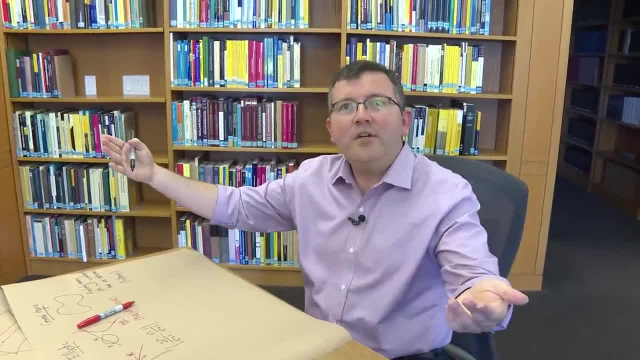 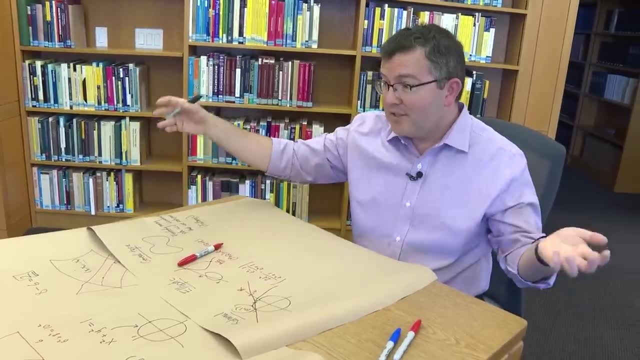 Exactly, Exactly. You can take a surface and just like, chop it up into lots of curves And then you know if you're looking for points on that give you a magic square of squares. One thing you might try to do is, instead of looking at the whole surface, just look at. 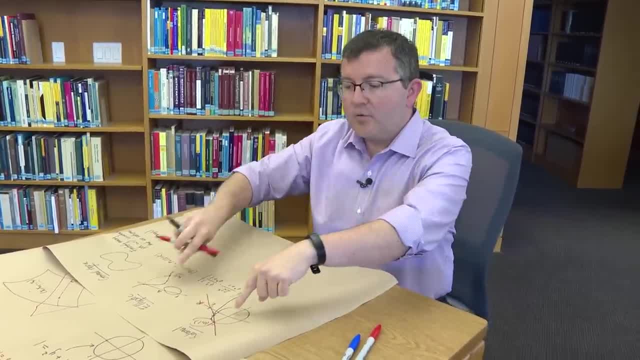 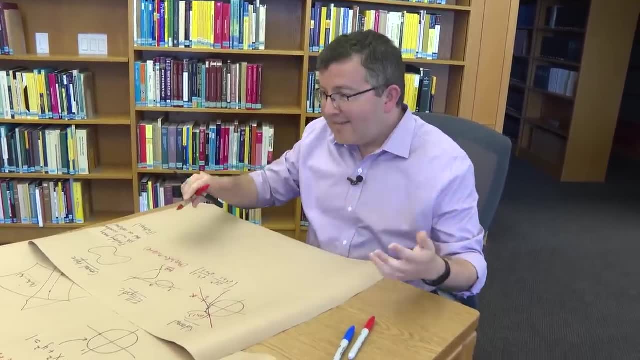 a curve inside that surface And maybe you get lucky and maybe your curve is one of these two types And then you can use what we know about these two types to actually construct magic squares of squares. But the sad thing is that the surface that parametrizes magic squares of squares the 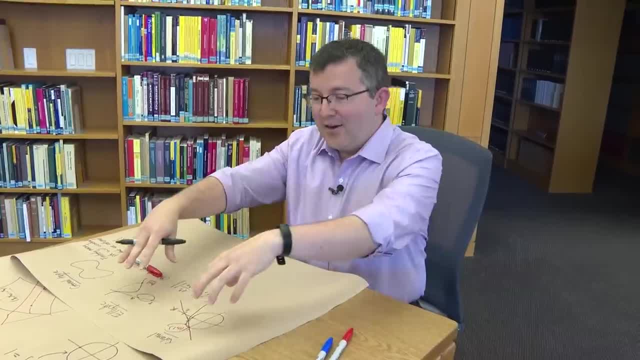 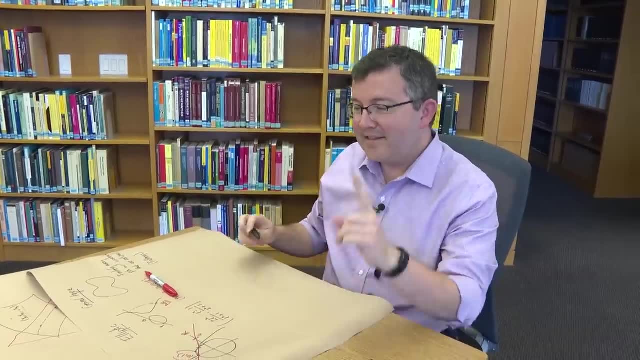 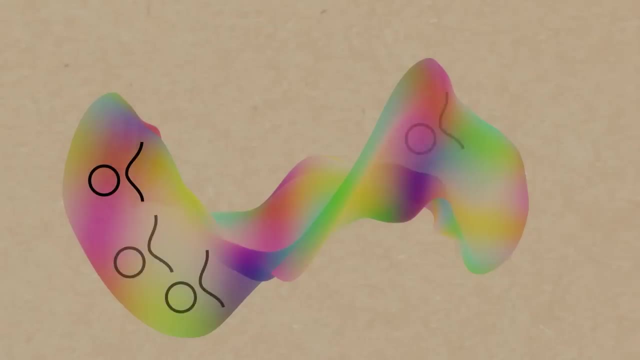 Parker surface has only finitely many of these rational or elliptic curves. It doesn't only need one. It only needs one, You're right. So here's the crazy thing: It has more than one. In fact, this Parker surface has 368 of these curves that we know of. 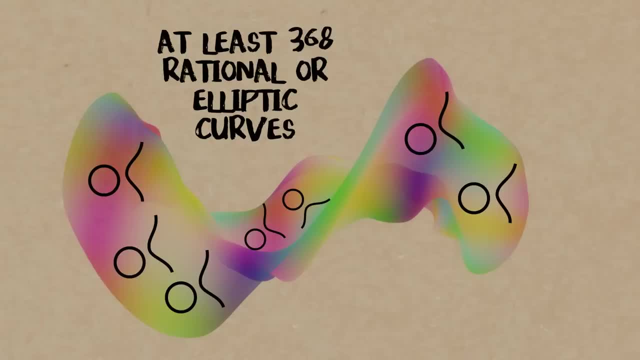 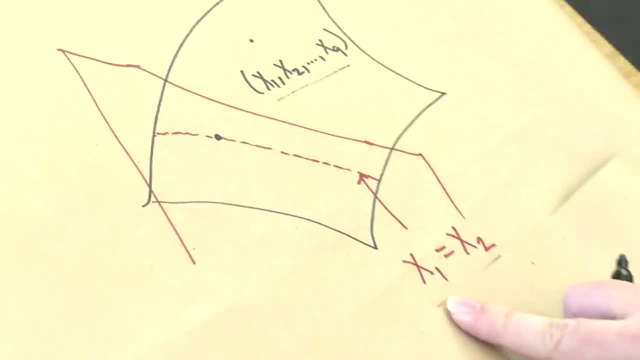 So there's at least 368 of these rational or elliptic curves. The sad thing, though, is that the way we've constructed these is that we looked at slices like this. You know what happens if I take x1 equal to x2, that gives me some kind of curve on. 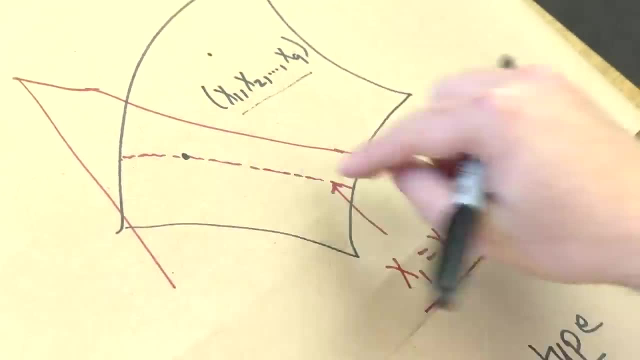 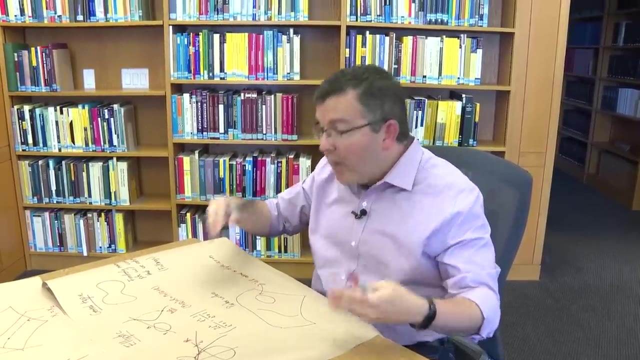 the surface, And then either this curve or, you know, the curve itself might break into a few pieces, Because when I do the slicing, you know those individual curves are either rational or elliptic, But they have this property that x1 is equal to x2.. 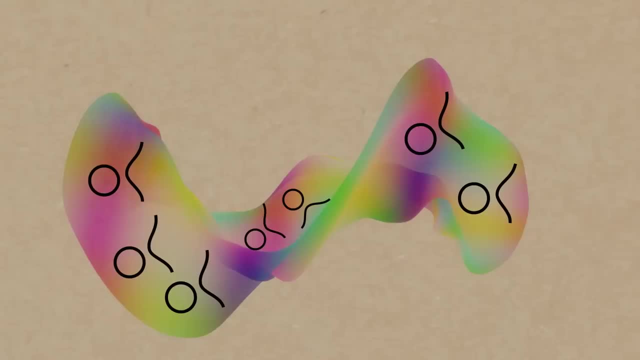 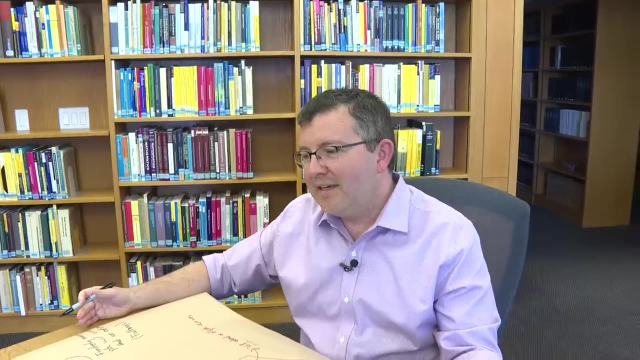 So the 368 curves that we can find. they contain points, But all of the points on these curves are going to give us these kind of fake magic squares, which is really, really sad. OK, And so here's the final kicker, though. 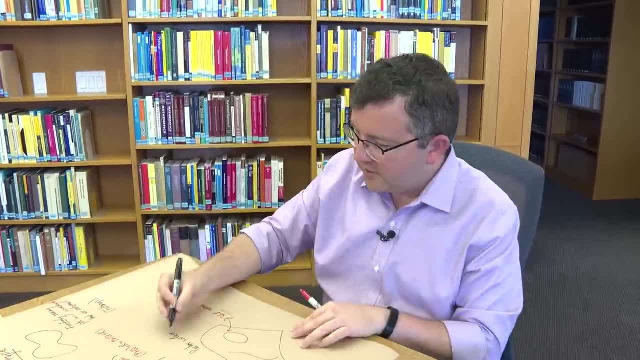 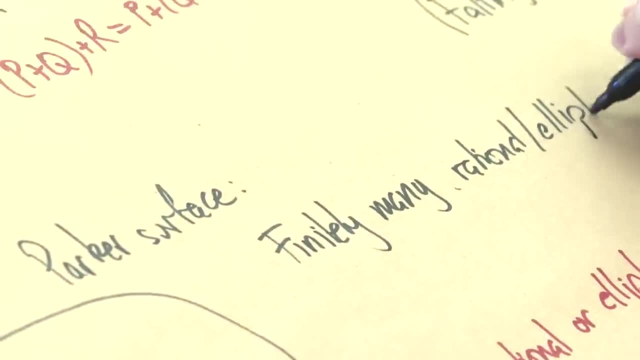 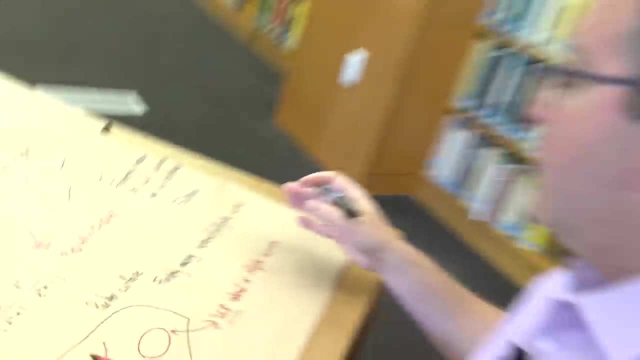 There is a conjecture. So Parker surface, So this has finitely many, finitely many rational and elliptic curves, So our idea to try to use these curves to produce points isn't looking so good. Like I say, this is some theorem that came out of work that me and a couple of co-authors 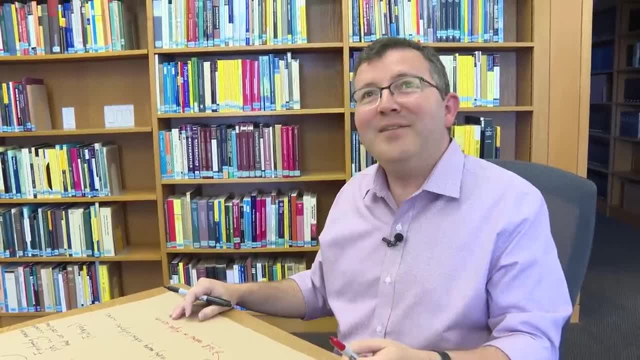 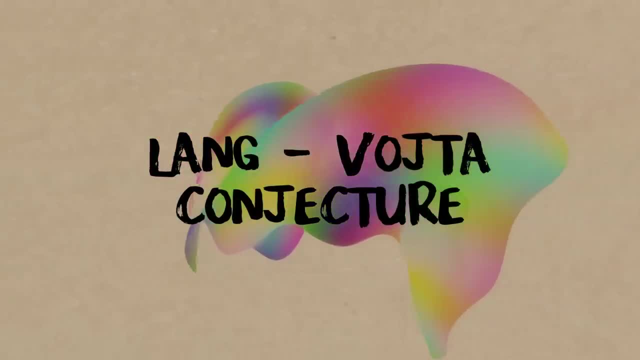 were working on And I mean it was kind of neat. We didn't expect that we would be able to prove something about this very specific surface. But now the kicker is that there's something called the Langvoida conjecture. This is the incredible thing. 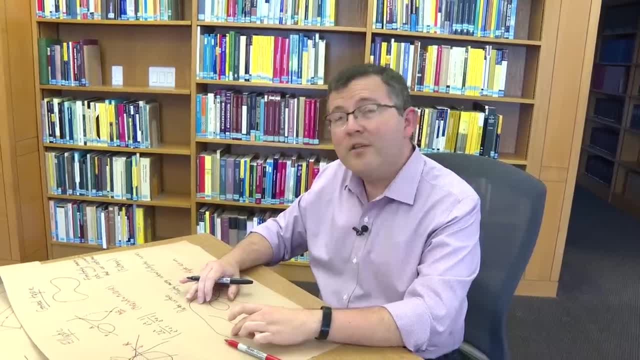 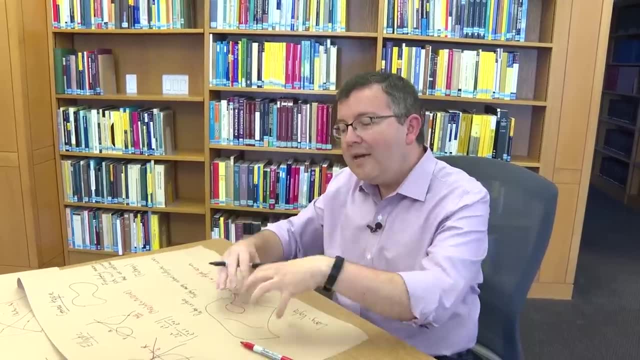 This surface that we have here is a particular kind of surface. It's also called the general type surface, And Lang and Voida sort of made a series of very deep conjectures. But when you apply those conjectures to the surface what it says is that outside of the 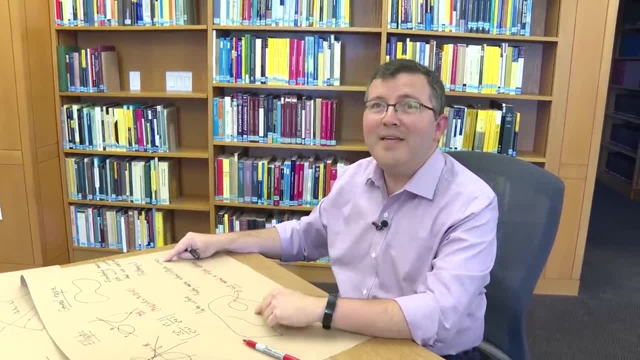 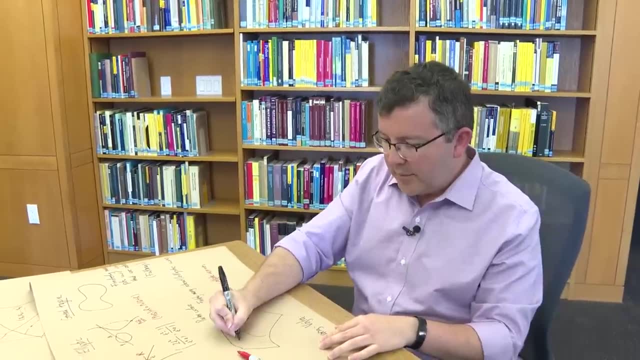 rational and the elliptic curves. there can be, at most, finitely many points on this surface, all of whose coordinates are integers right. There's tons and tons of points on the surface, but there's only going to be finitely many. 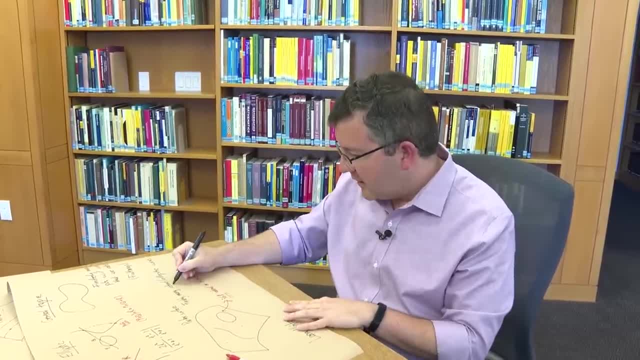 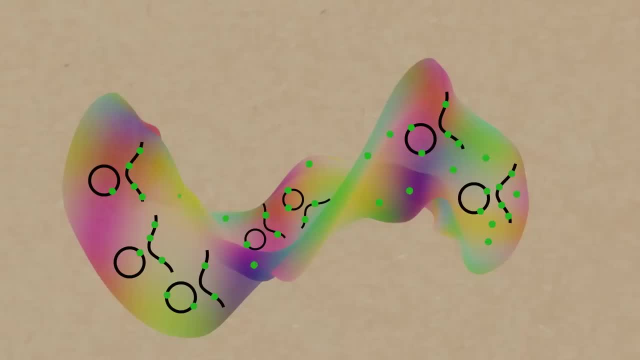 points Outside of this nice locus of rational elliptic curves, all of whose coordinates are going to be integers. There's finitely many- I'll call them rational points outside the rational and elliptic curves. So where does that leave us? 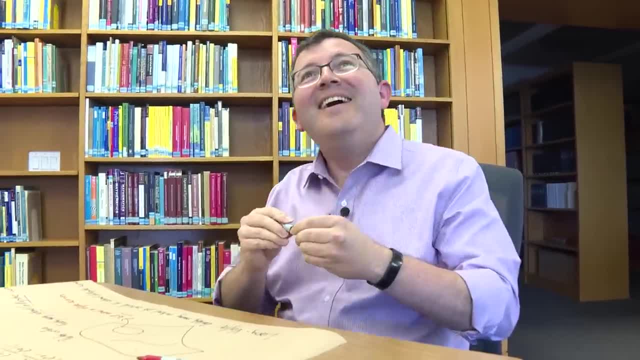 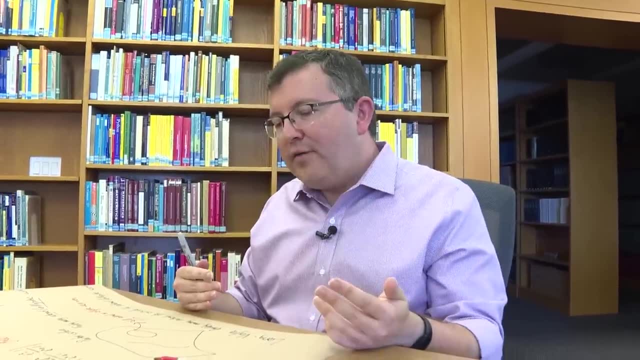 I get the feeling from talking to you: as soon as a search space becomes finite, you become very despondent and lose hope. Yes, It's finite because of this sort of general conjecture. But often finite can mean empty as well. 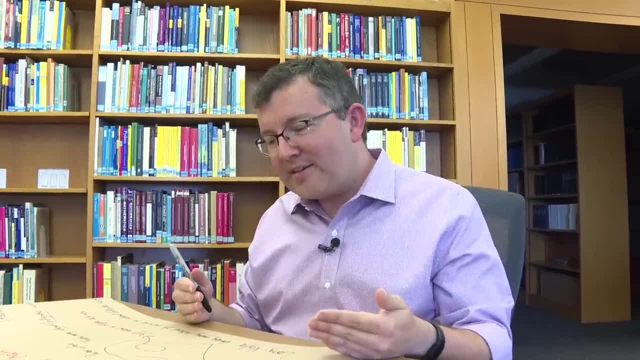 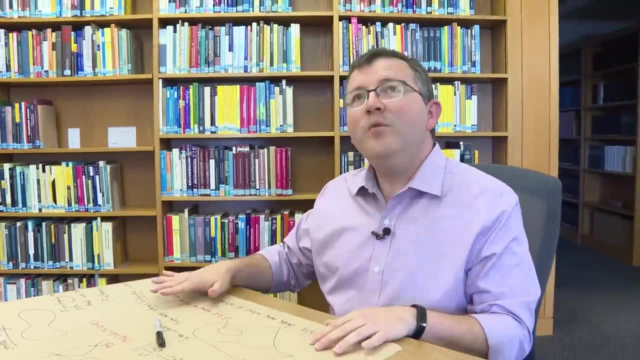 And so it's entirely possible That it's not just finite, It just isn't there. There just isn't a set of points. So somehow the moral of this story is that either we need to find some more of these rational or elliptic curves on the surface and hope for the best. 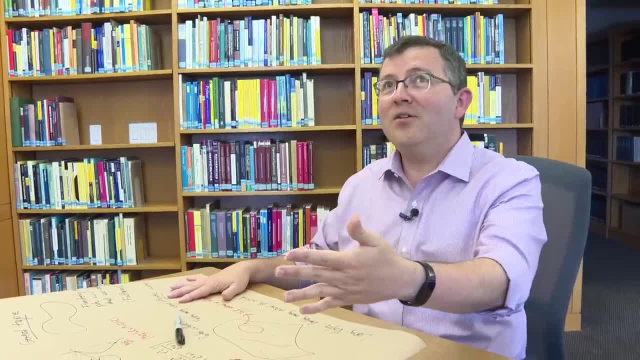 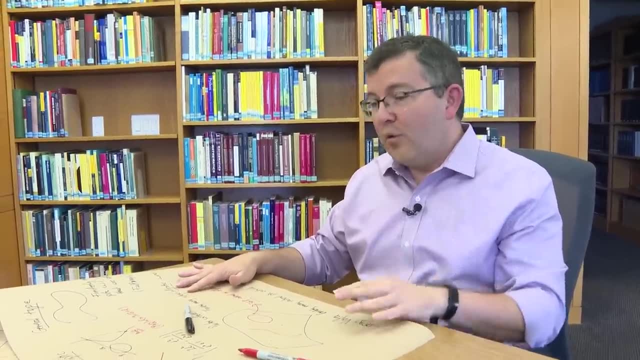 There's only a finite supply of them, so we can't just keep trying this all the time, And in fact we might actually get a complete list at some point of all of these, And then we really understand points on rational and elliptic curves. 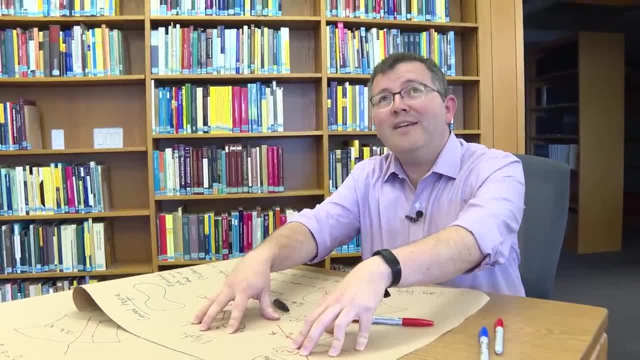 And then we might actually get a complete list at some point of all of these, And then we really understand points on rational and elliptic curves And then we really understand points on rational and elliptic curves. So once we have that finite list, final list, we'll be able to ascertain whether you get. 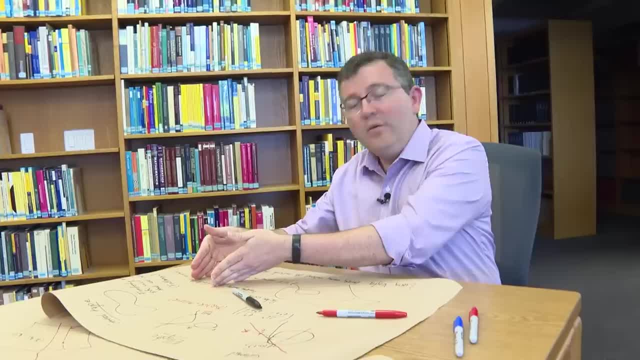 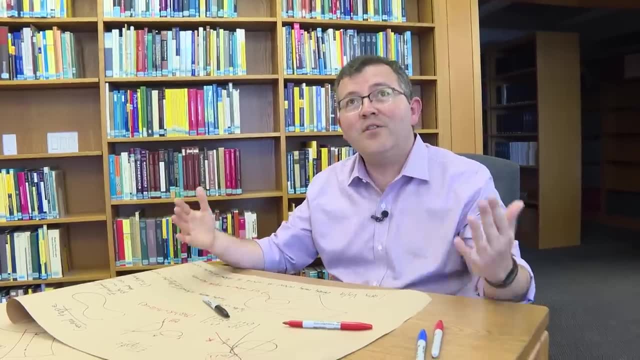 one of these magic squares of squares, at least sort of from that point of view. Or the other hope is that well, we do this and we find nothing, But somehow there's this miracle And for some reason that we just don't understand. 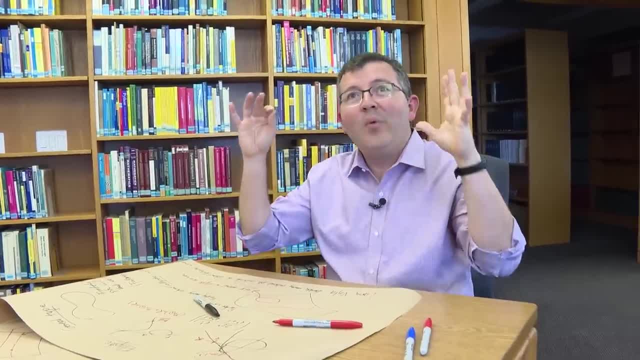 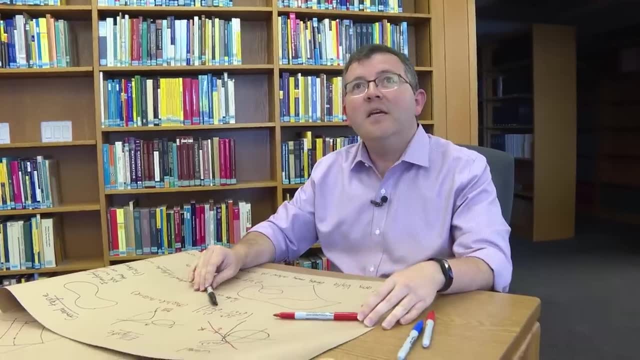 There's a couple, one or a few more sporadic points on the surface, all of whose coordinates are integers, But everything we know about the geometry of surfaces And the geometry of curves is really pointing to the idea that there just isn't a 3 by 3. 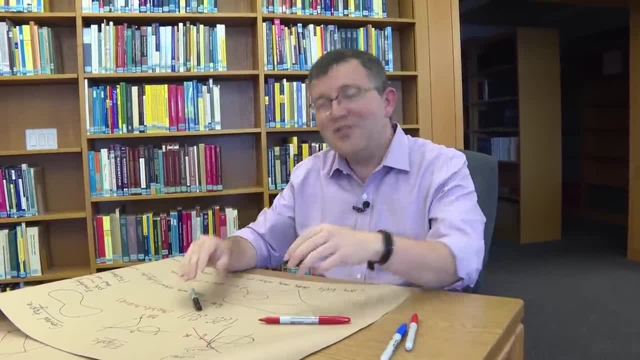 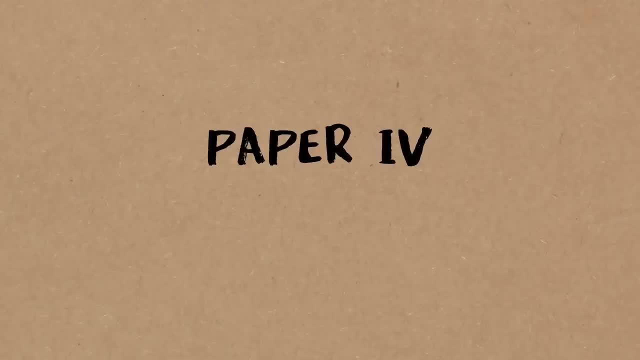 magic square of squares in the way that we would like it, with distinct integer coordinates, which is kind of sad. But I want to end on a good note, though, so I need one more piece of paper, So what I want to show you is something that's kind of mind boggling. 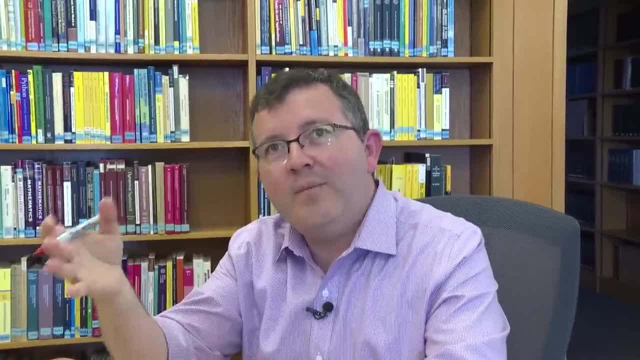 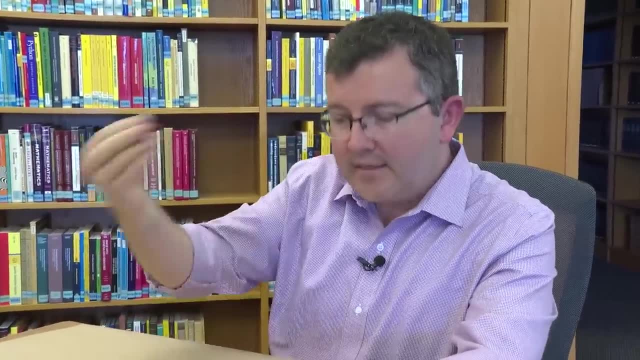 So we've been asking for magic squares of squares, which were 3 by 3, grids that had this property that the columns, the rows and the two diagonals added up to the same thing And all the entries were squares. OK, 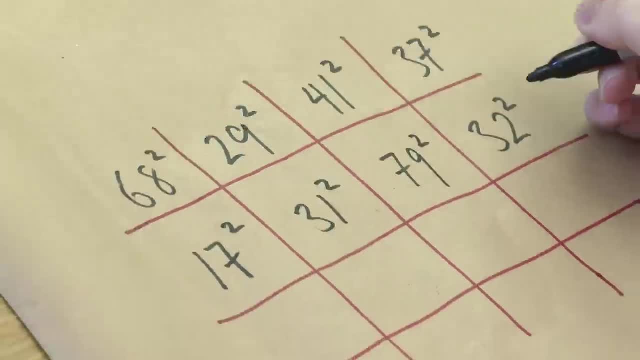 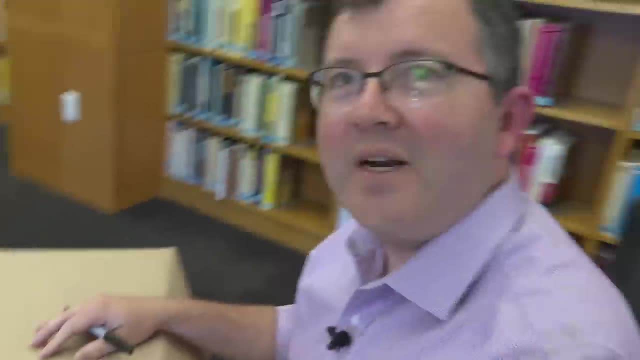 But now you can do, we can go for broke here. You've got a 4 by 4 now. You've got a 4 by 4 now, And this is kind of amazing, OK, So this is a 4 by 4 magic square of squares. 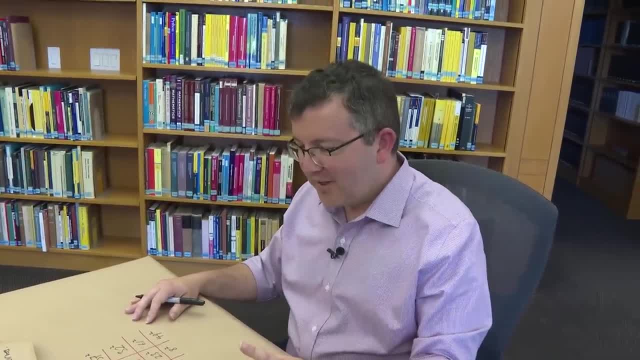 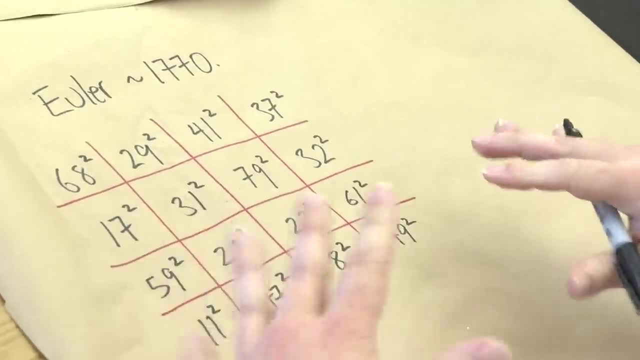 This is not a fake magic square of squares. This is the real deal, Due to Euler around 1770, thereabouts. these magic squares of squares have a very long history. If you look here, sort of all the rows, all the columns and the two diagonals add up. 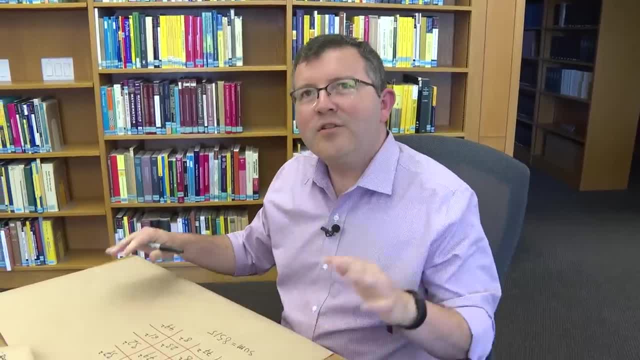 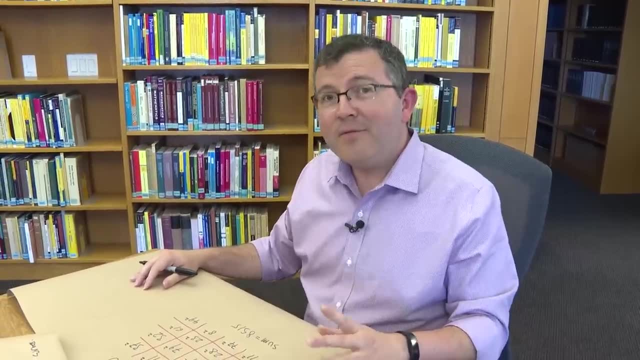 to the same number, 85, 15.. So this is kind of crazy. You know there's a 4 by 4, but there isn't a 3 by 3.. OK, And if you go on the internet, you'll also find a 5 by 5, and a genuine one, not a fake. 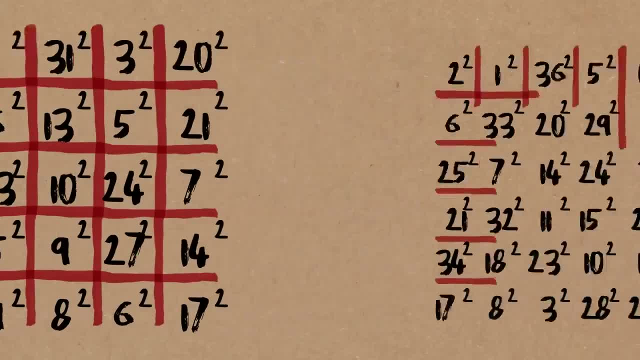 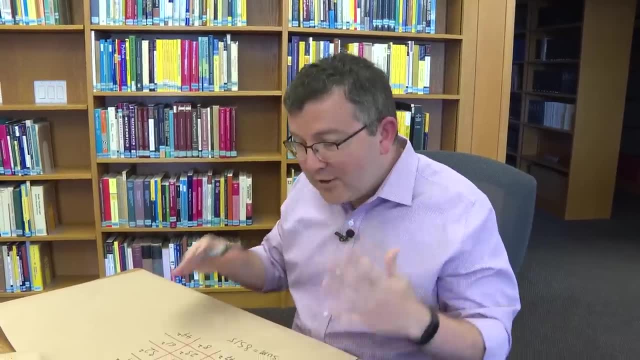 one, You know, like we. and if you dig far, you know there's also a 6 by 6, and so on. From the geometry point of view, this is actually not too surprising. In fact, I would actually think it would be really cool to show that if you take an n. 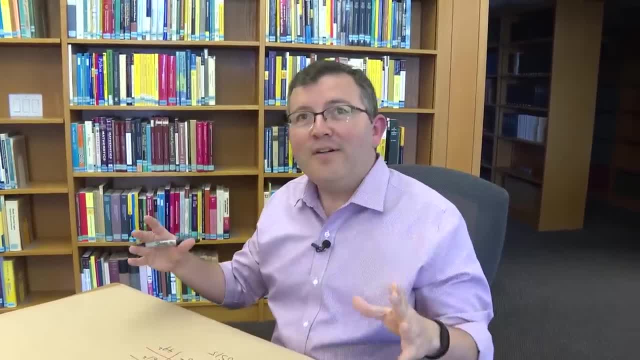 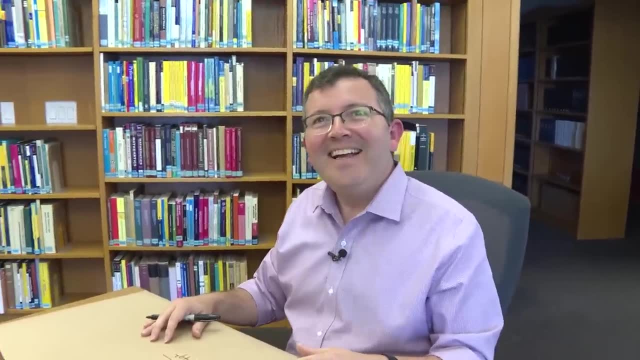 by n grid, then, and n is at least 4. Then you can produce one of these magic squares of squares. And so what happened when you kicked up? because I thought, if you applied when you, I thought, if you applied that same process, you just showed me right to this- you'd. 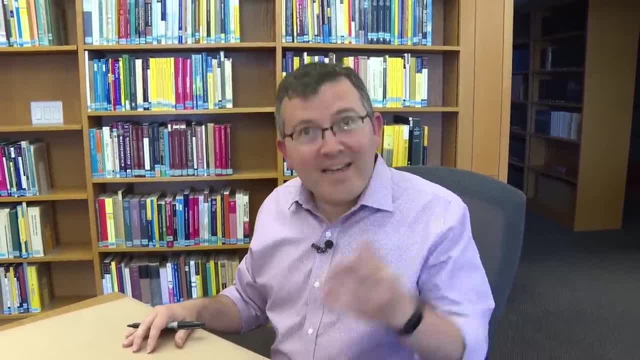 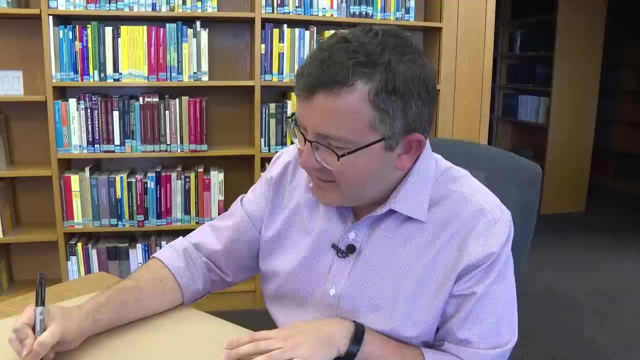 have the same problem, You'd come up with a surface that was really constrained, Exactly OK. So what happened, Right? So let me just sort of explain briefly, Right? So if I have like an n by n grid, right, that means that I'm going to have something. 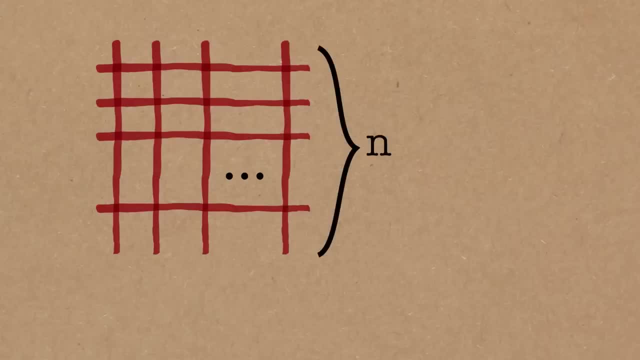 like what we did before. So this is n entries this way and n entries that way. OK, So if you have an n by n grid, you have n rows, you have n columns and you still only have two diagonals, OK, 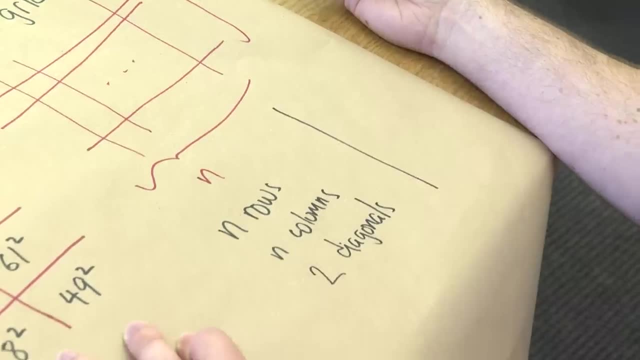 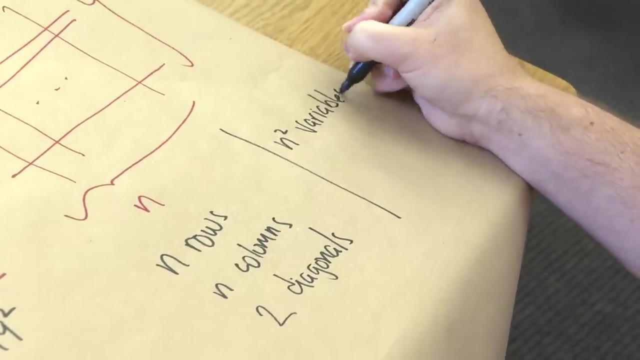 But now, OK, how many variables do you have? Well, there's n times n, So there's n squared variables. So in the 3 by 3 case there were 9 variables. In the 4 by 4 case there were sort of 16 entries. 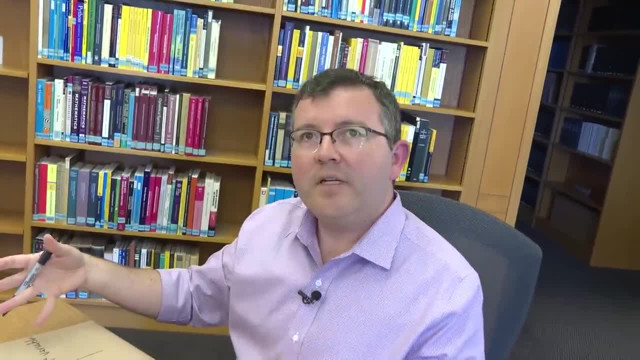 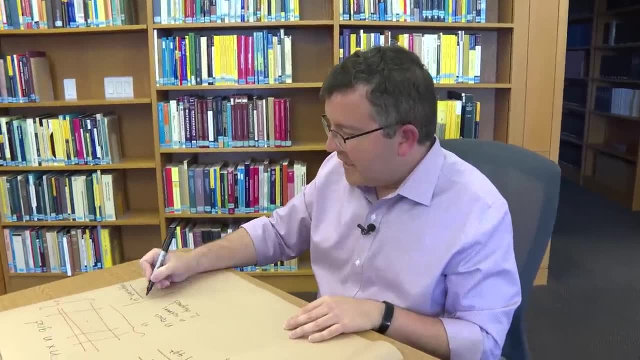 So if you were on an n by n grid, there's going to be n squared variables. OK, So what has happened here is that The space in which we're working in right, the number of coordinates that we're going to need, is growing really fast. 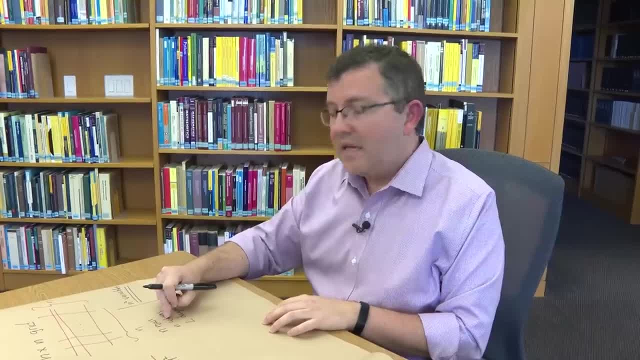 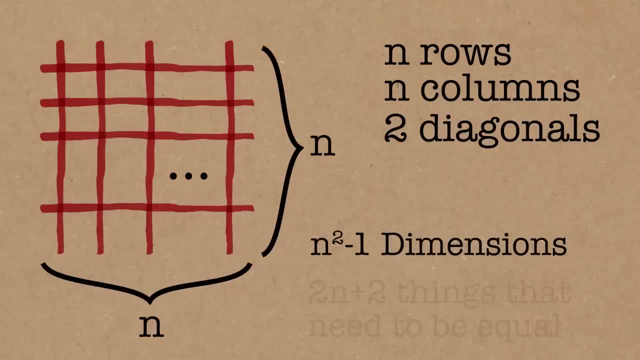 But the number of conditions that we're trying to impose on that space is not growing anywhere near as fast as the space itself. So the space itself has dimension n squared minus 1.. And then I have 2n plus 2, things that I need to set equal to each other. 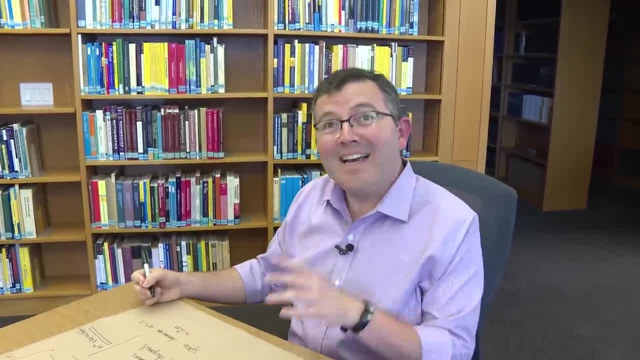 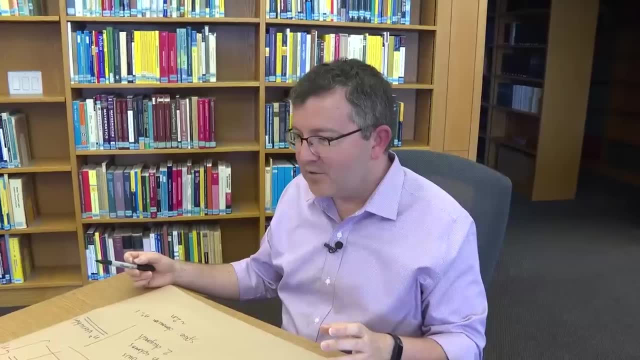 So the Parker surface is no longer two-dimensional? Exactly, It's no longer two-dimensional. It's like a huge blob. Exactly, It's like a huge blob, right, We go up one dimension to n equals 4, right? And now we're in 15 dimensions. 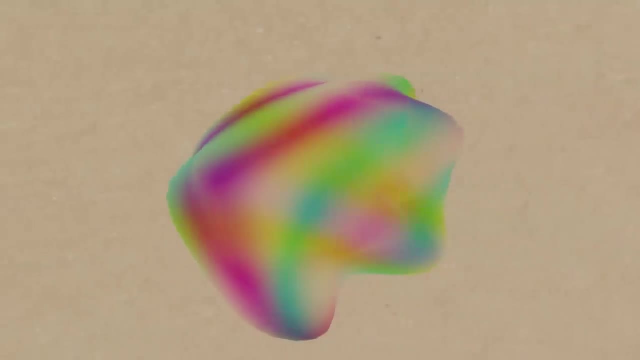 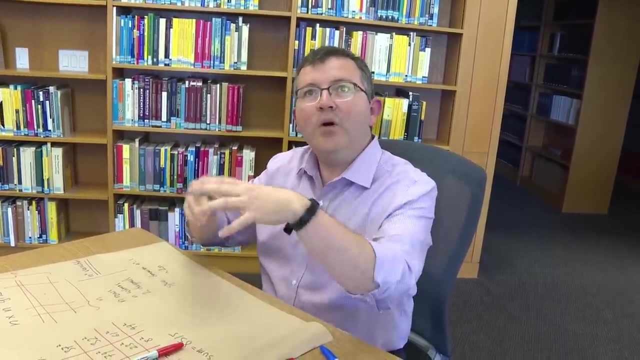 We've made roughly 8 huts, And so it's like a big blob. It's not a surface anymore. Parker blob- Yes, That's right, The Parker blob in n dimensions, And so the cool thing, though, is that these sort of conjectures that we have about points 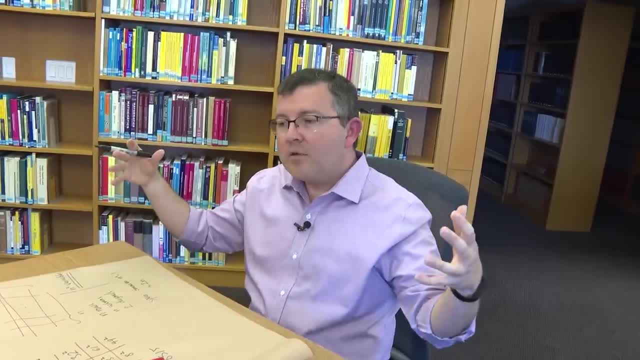 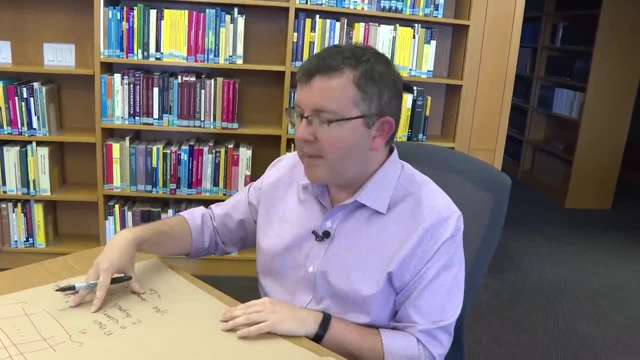 on these blobs. right, It's not a surface anymore, It's a much bigger blob, And so things get harder and harder as these dimensions go up. But the main point is that The main point is that the geometry of these spaces: as n grows, it actually becomes more. 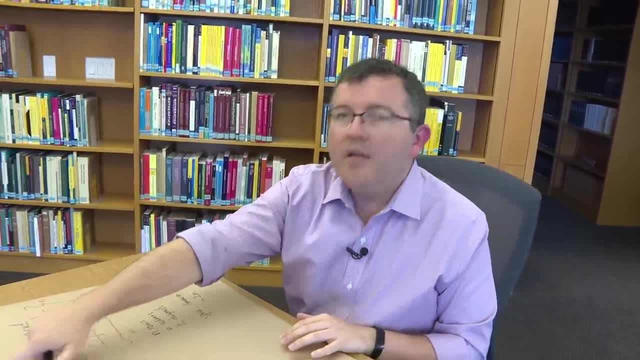 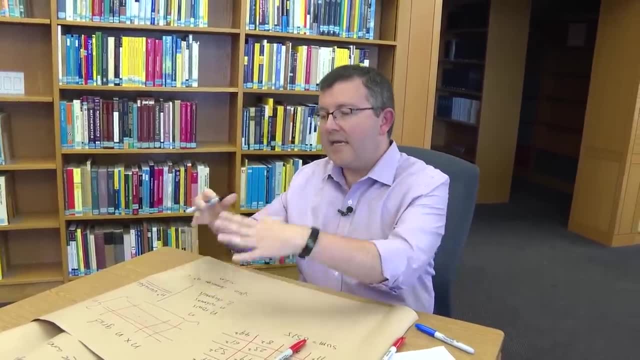 positively curved, which means that it can harbor tons and tons of these kinds of rational and elliptic curves. And so, in fact, for blobs of this kind as n grows, we actually suspect there are lots and lots of points on those blobs. 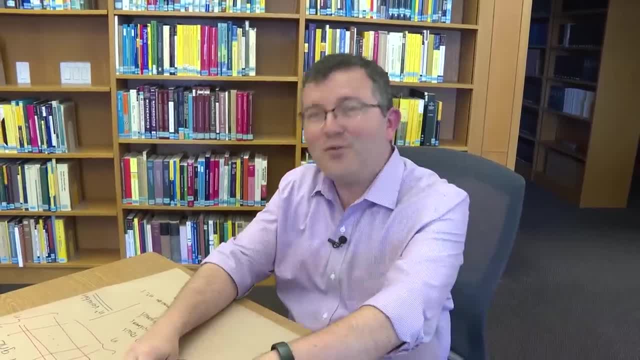 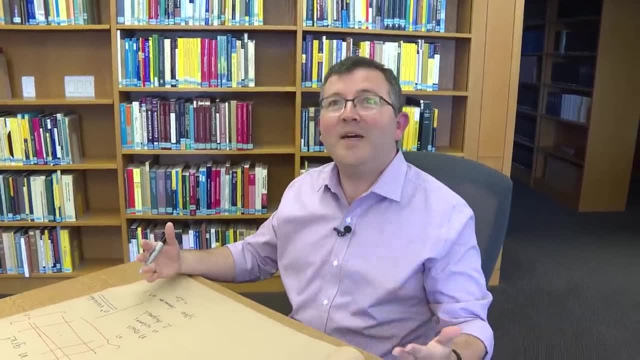 And so it's sort of not too surprising from the point of view of geometry that you would find a 4 by 4, magic square of squares, or a 5 by 5, or a 6 by 6.. You know, It would be really cool to prove that you can get an n by n for n at least 4.. 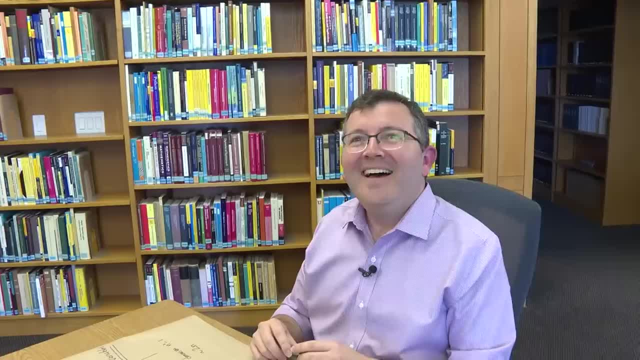 Now do you know what would be cooler? Just finding some number out there, n by n square where there isn't a solution again? Oh my God, That would be amazing, Like some freak curve. Yes, That's right. 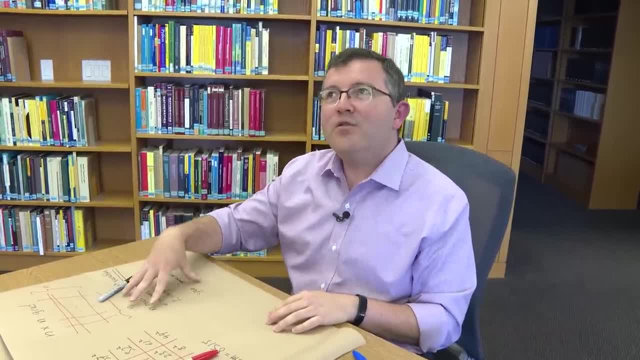 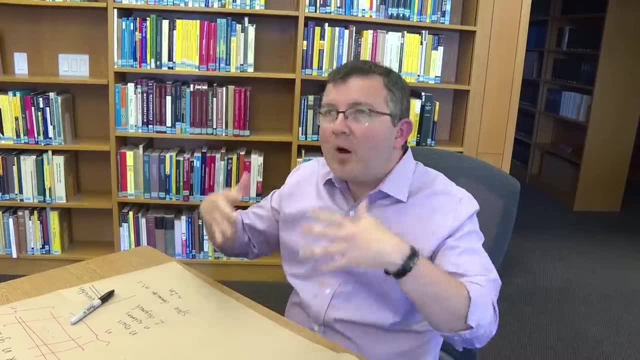 And that could happen, Because you know, in fact these spaces are very singular And so sort of the notions that we have about what ought to happen may or may not work in those spaces. I mean, we sort of think that probably it's going to be okay, but we don't really know. 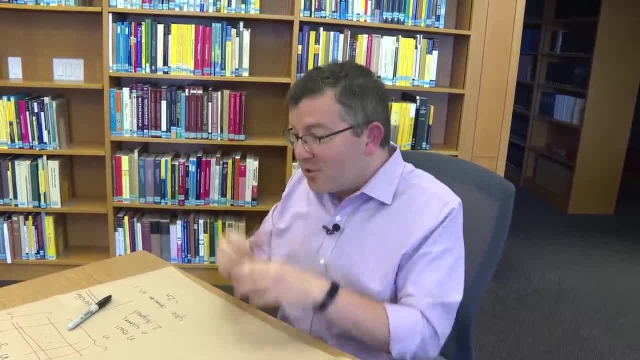 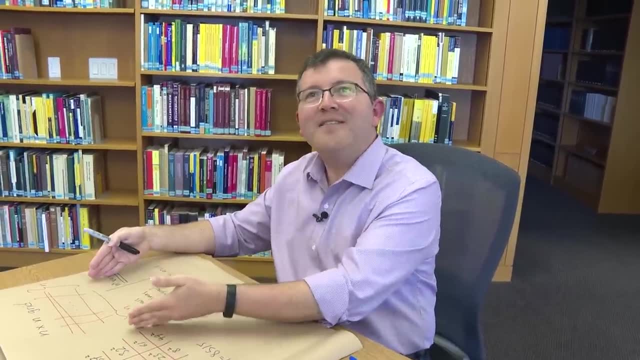 And no one has really sort of sat down to explore these spaces. Yeah, There's some really interesting mathematics. You know, at first it might seem like, oh, we're just having some fun with squares, But there's some really deep geometry that's going on behind the scenes. 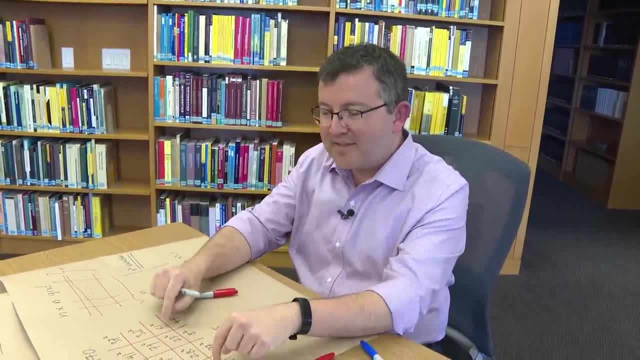 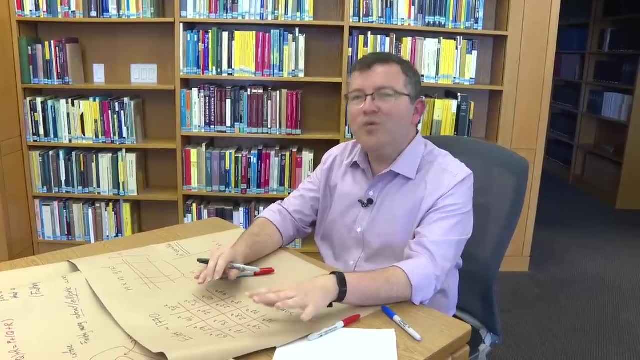 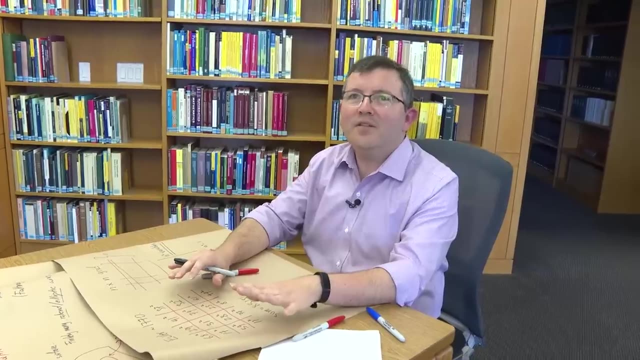 And in fact I can't resist saying this. but this square that Euler came up with is really important in the proof that every integer is a sum of every natural number is a sum of four squares. There's a very famous theorem of Lagrange. 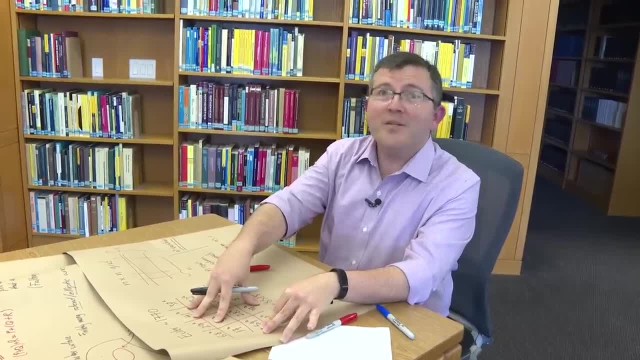 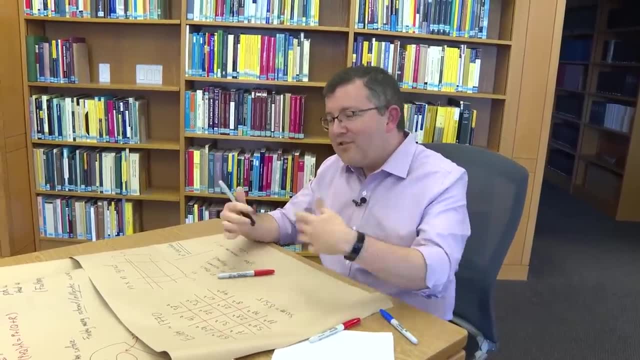 In fact, Euler sent this particular square to Lagrange with no explanation about how he had constructed it. you know, And then you know, Lagrange had to kind of work hard. And then, you know, Euler eventually did publish the method. 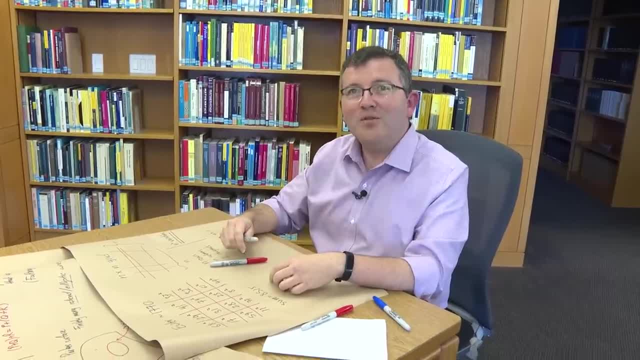 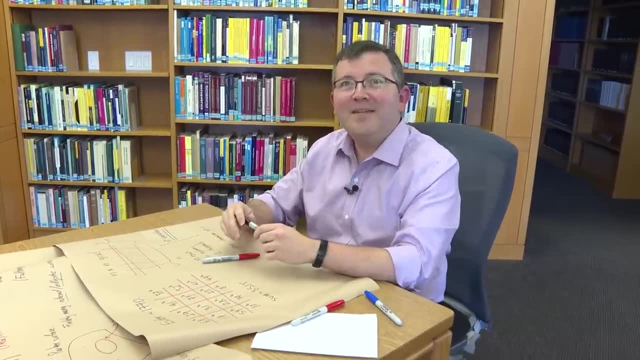 And then once Lagrange saw what Euler was doing, you know he was really able to complete his proof. But it's amazing to me that sort of this that might seem just like pure fun actually ends up having some really sort of deep and interesting consequences. 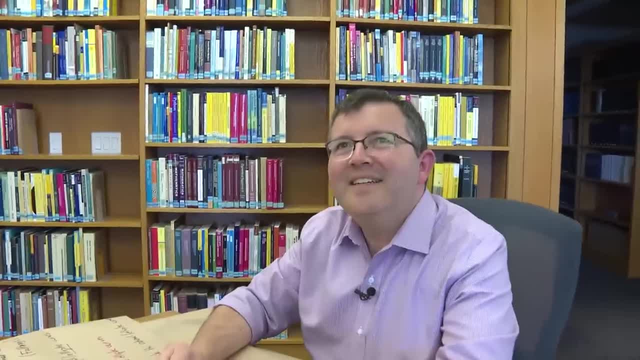 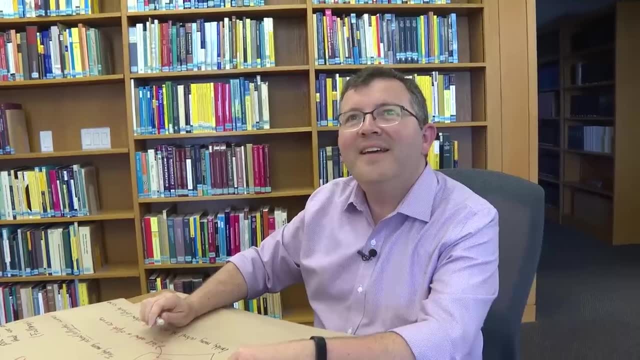 If you find all the finite curves on there, Yeah, Rational and elliptic, Yeah, Yeah, And they don't throw up what you need, Can you prove that there are those? can you prove that there are none of those other points floating out there? 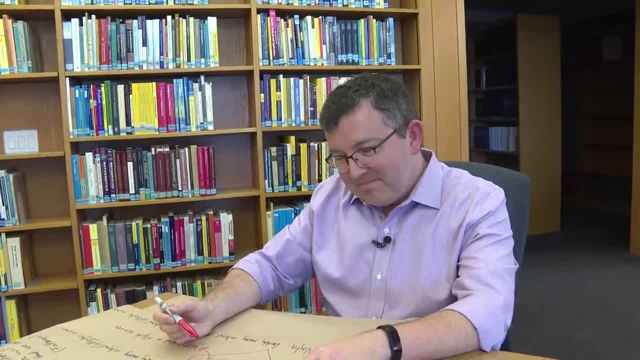 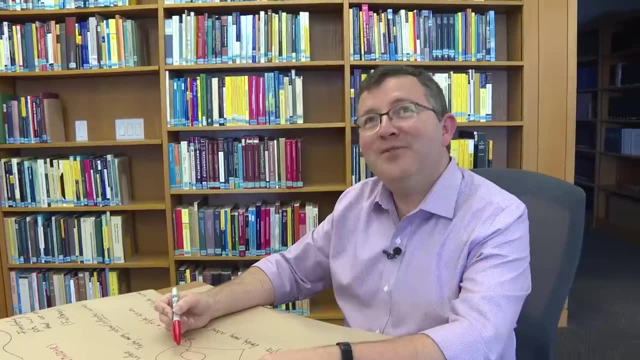 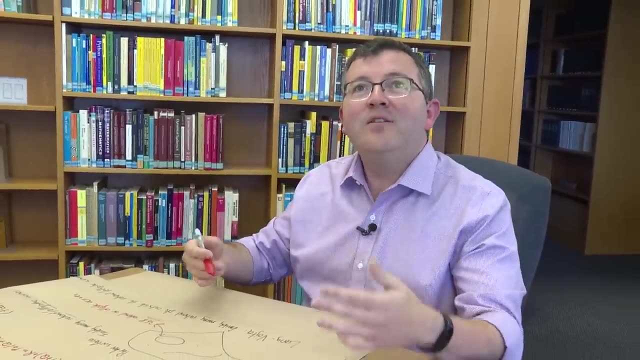 Is that provable? Can you say yeah, there aren't any points as well? Or are they always going to be a bit of an unknown With current mathematical technology? I would not know how to do that, And I think that that's sort of in general. it would be great to have some kind of mechanism.